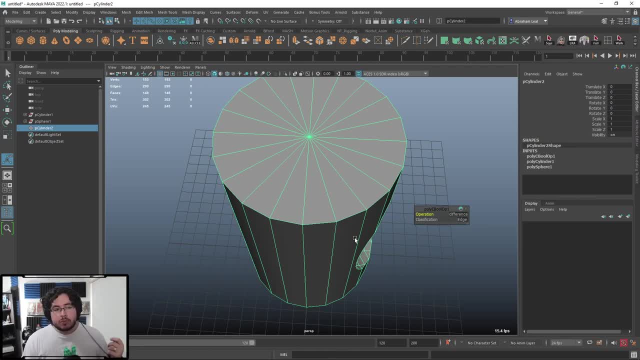 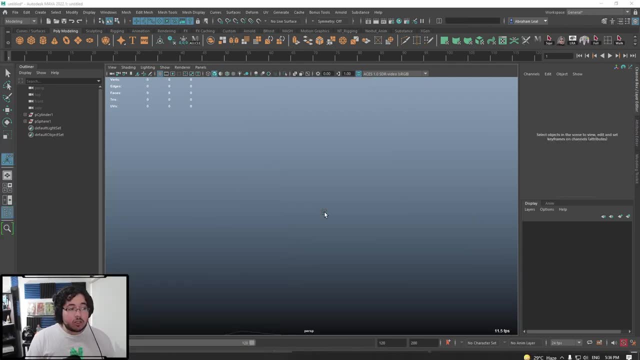 are usually not that good, And the reason why they're not good is because, as I'm mentioning here, the topology is just really, really bad. Now, that does not mean that booleans are our enemies, because there's actually ways. I'm going to show you here in ZBrush one way. 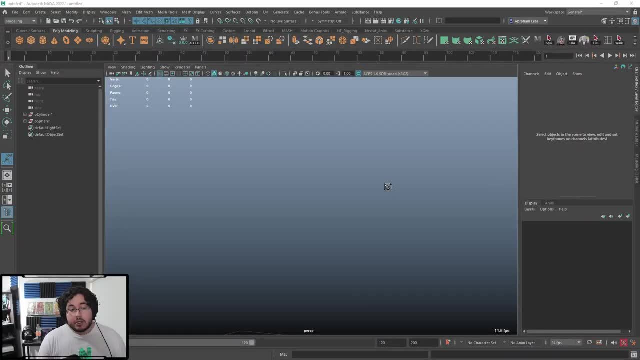 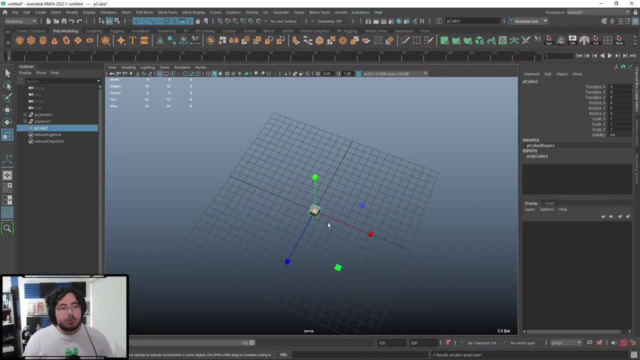 in which we can actually utilize booleans to our advantage to create some very nice shapes. Now, the most important thing that you need to know is that booleans are really really good shapes. What you understand about booleans is that they will give you the shapes that 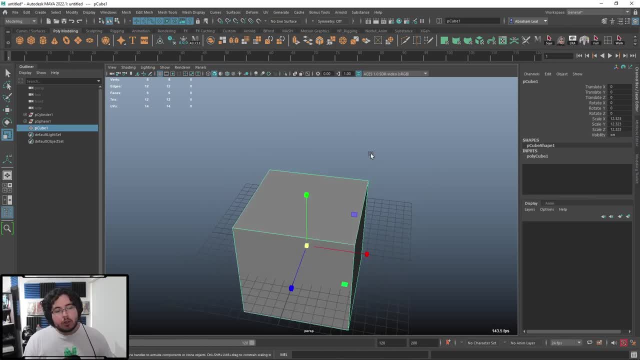 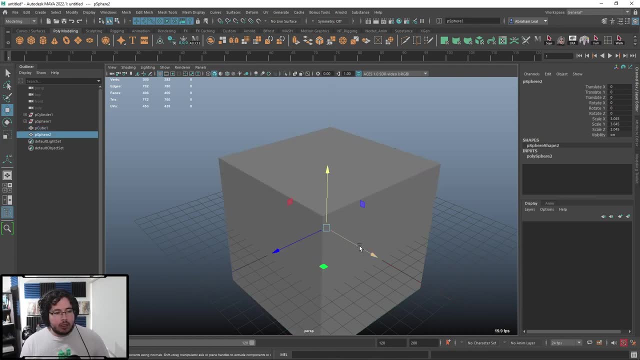 you're going for, But unfortunately, those shapes are or might not be exactly the shapes that you want to use in a game or in subdivision modeling, And the main reason is, when you use a boolean, as you saw with the previous example, what's going to happen is you are 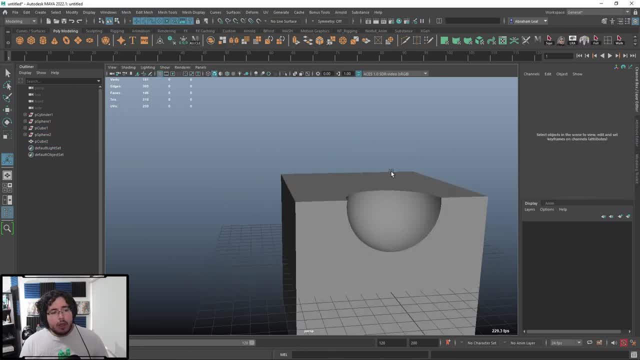 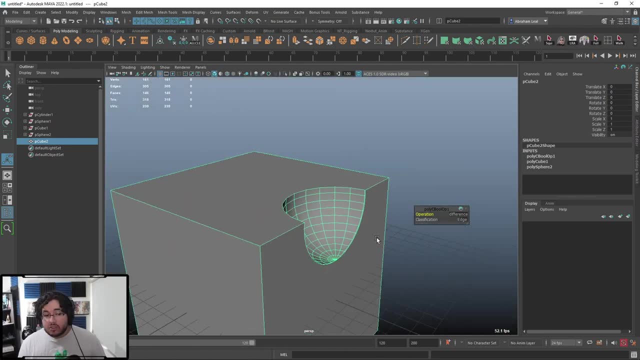 going to subtract, as you can see here, one object from the other one And, yes, you'll get this very, very nice effect, But unfortunately this is non-workable. geometry Like this geometry is not something that you're going to be able to use anywhere. 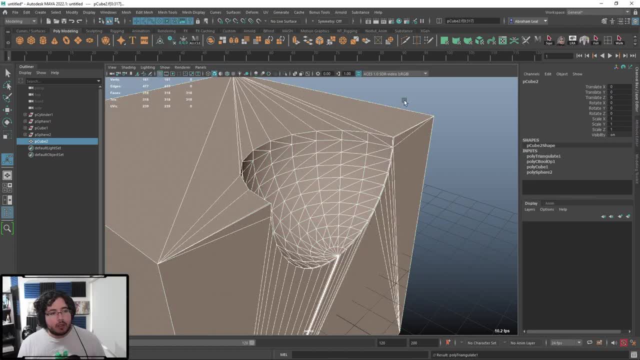 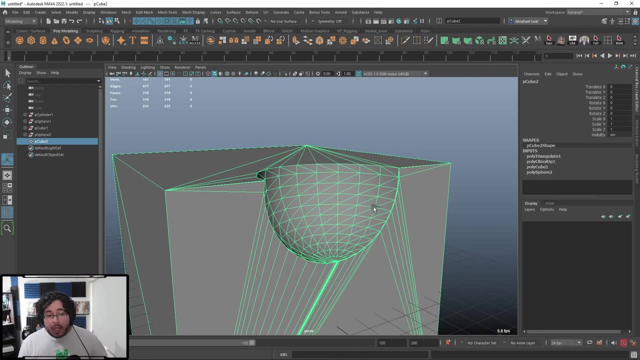 Unless you just want to like 3D print this thing and you're just going to triangulate and that's it Like. if this is the shape that you want to 3D print, then go for it. Like, this is perfectly fine, It's perfectly workable. However, if you want to use this for games, 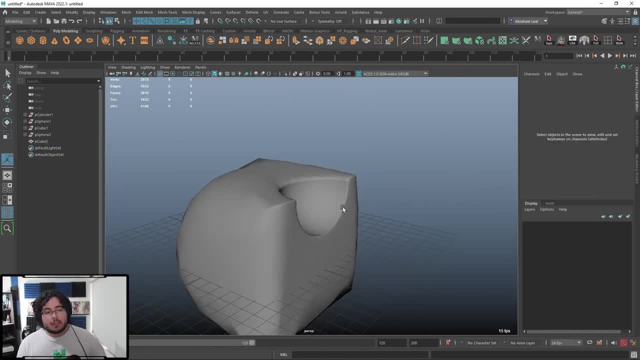 or, if you want, to use it for subdivision modeling. as you can see, when I subdivide, we get this super, super ugly element. So some of you might be wondering: well, does that mean that booleans are bad for us? And the answer is no. They can actually be very good, but you 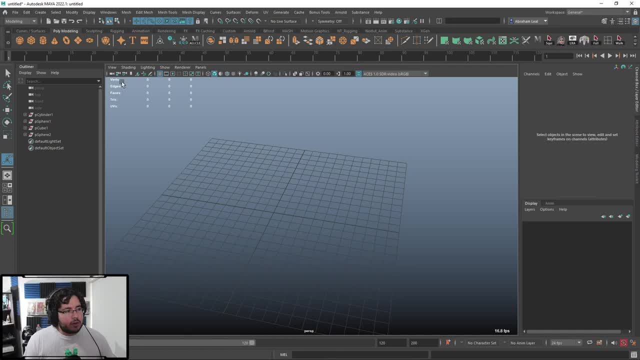 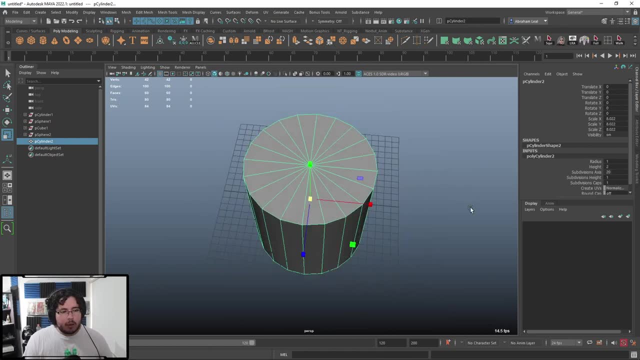 need to know how to properly do them. Okay, So I'm going to show you here an example. This is something that I teach my students in my first like a modeling class. This is when we have like a just like an average thing And we're going to be doing. 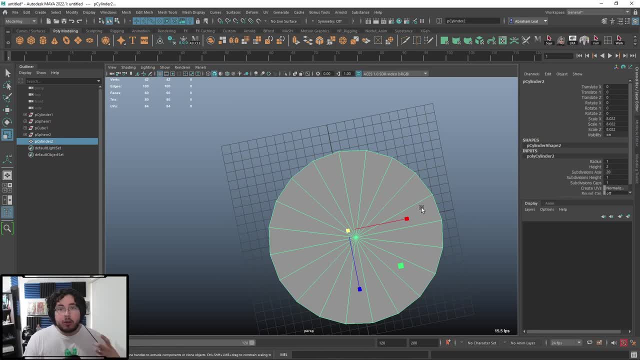 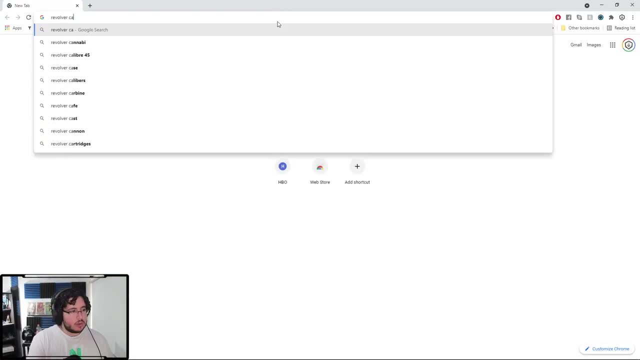 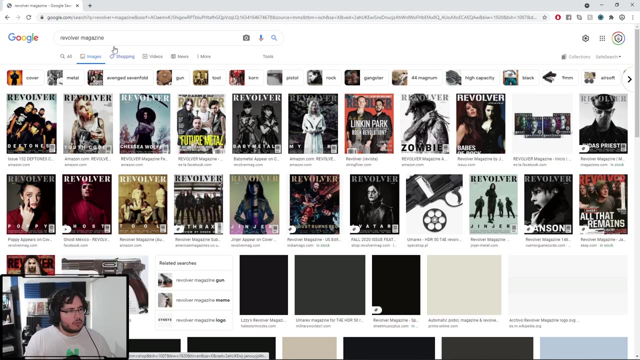 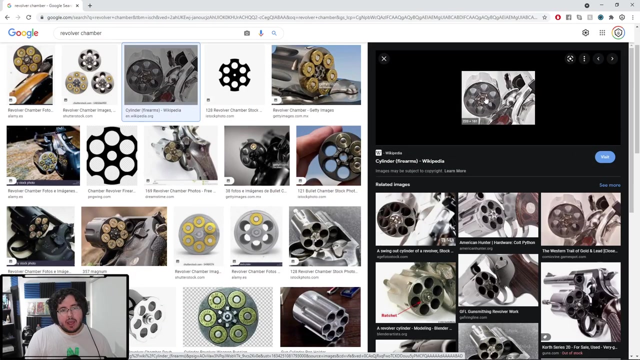 very quickly: a like, a like a revolver barrel. So everyone has seen the revolvers like magazine, revolver, magazine, And it's this sort of a round shape, right So revolver chamber, Is that it? There we go, So this sort of thing, right, So we have six holes throughout the 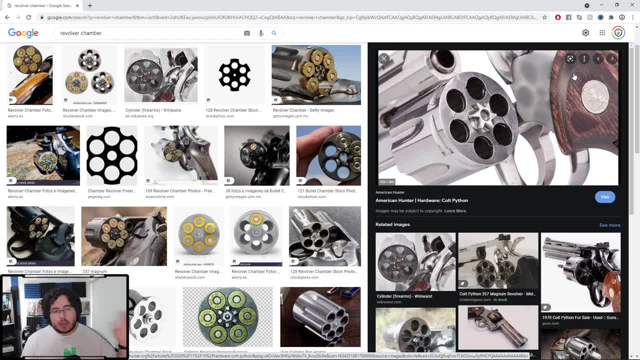 thing And then we have this very nice like a smooth things Everyone. there's a lot of people out there that have been doing tutorials showing you how to how to model guns and stuff. We're probably going to do a a a modeling gun tutorial later on, But for now I'm just going 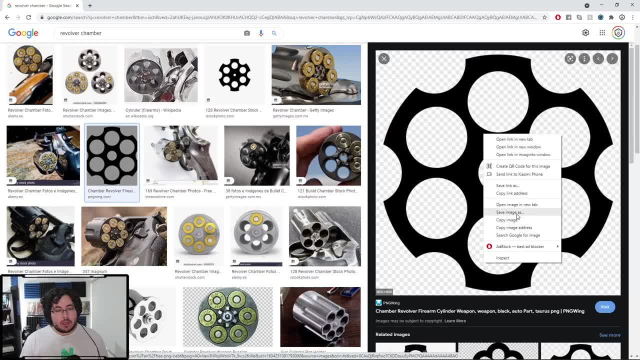 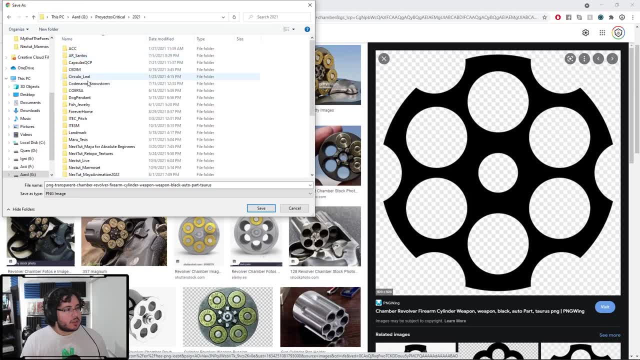 to show you how to do this real quick. So what I'm going to do is I'm actually going to grab this guy right here. I'm going to save this image, I'm just going to place it on my. let's go on next to live. We already have our project, So why not? So let's very. 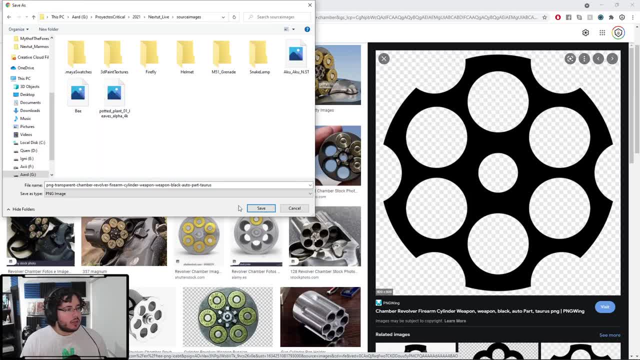 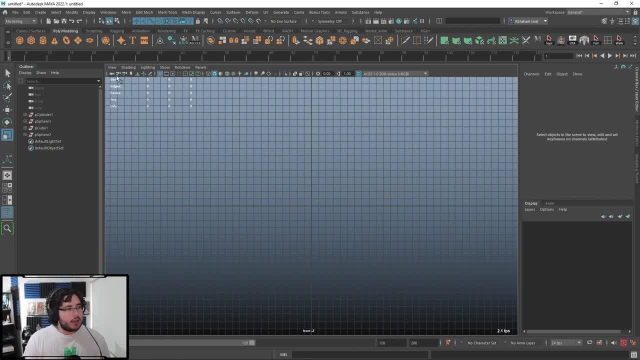 quickly go here into next to live and in our source images. I'll just save this right there And then here I'm going to go to, I'm going to go to my front, view, and I'm going to say view, image, plane, import image. 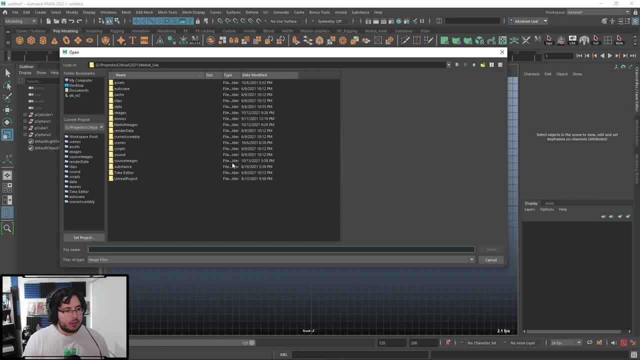 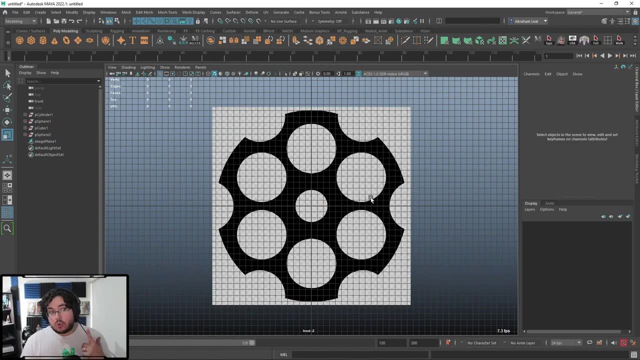 We need to set the project, of course. So next to live, there we go, Set, And from our source images, we're just going to grab this one right here. There we go. So this is the shape that we want to create right Now. the first thing that you need to understand is: we could. 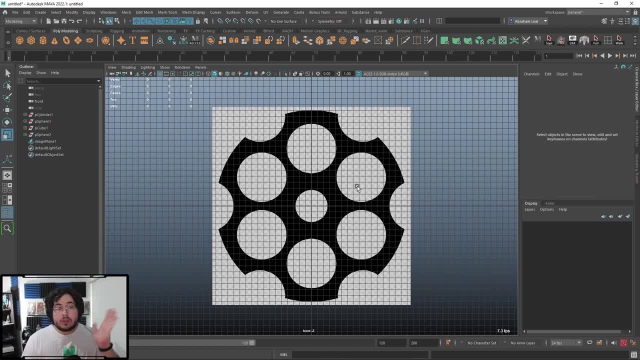 save ourselves a lot of work by doing this in a sort of a mirror way, right? So if we were to create- think of it like a pizza- So if we were to create like a, like a, like a section of the pizza, right here, it would be very easy to just duplicate around. 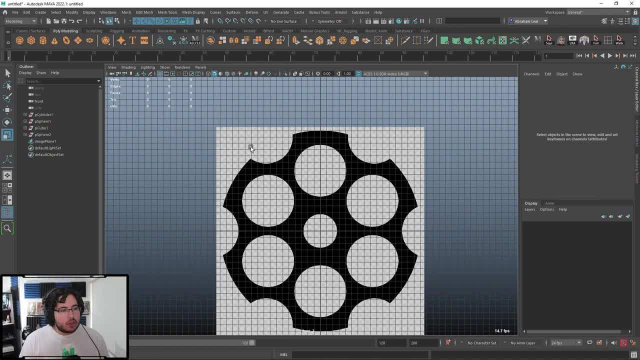 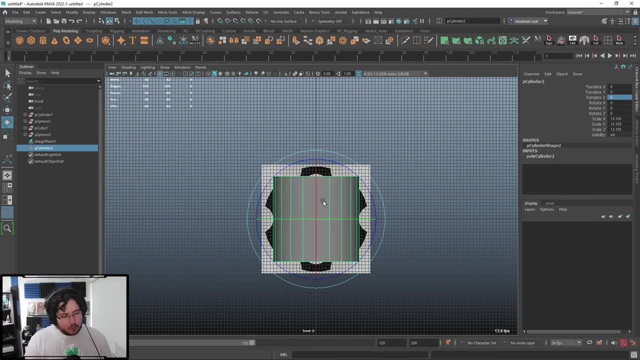 So we don't need to do the whole thing. We can just focus on one of the of the elements. So I'm going to start with a cylinder here. It's going to make a very big cylinder Rotate this 90 degrees. Remember we have- I've mentioned this before- If you press E and click you're. 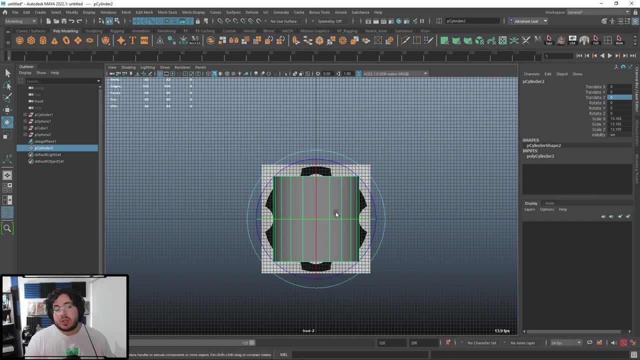 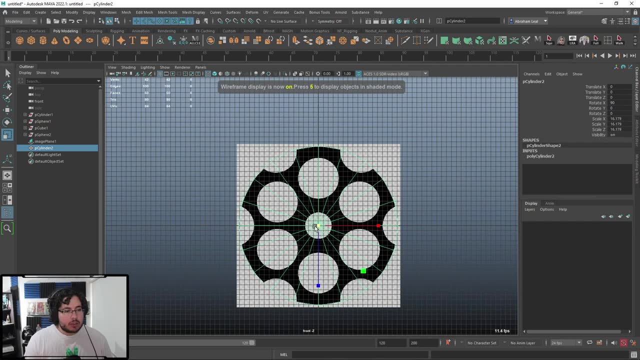 going to go into the options for the rotation tool and you can go into this discrete rotate and that's going to rotate in angles. So it's easier to just go into 90 degrees so that you don't have to type it in every single time. So I'm just going to make this this. 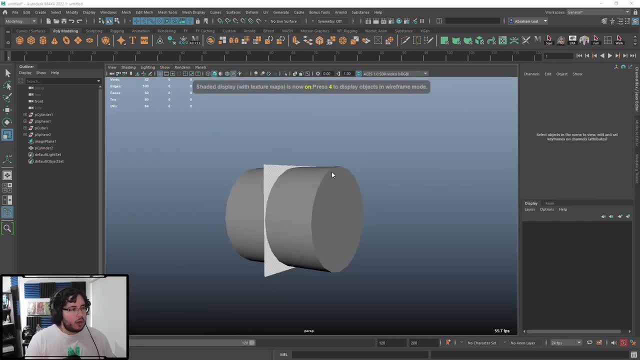 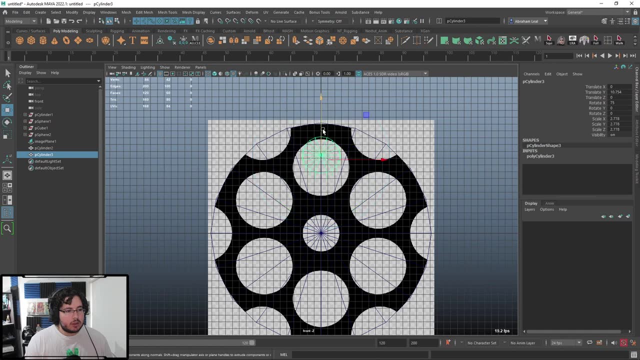 way. So now that we have the basics, that's perfect. Now let's just create another cylinder which is going to be the hole for the element. Again, 90 degrees, And we're just going to like modify this. Let's do 90 degrees, And then we will just like modify this so that it fits right. 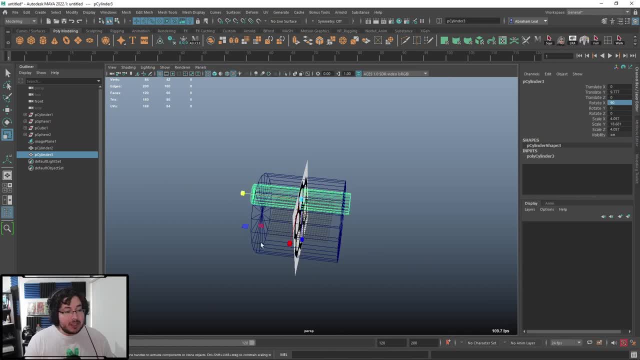 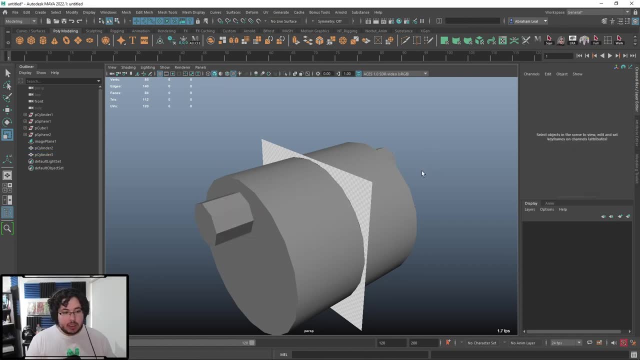 there And some some schools, some like people, teach students to just go and do it like a bullion here. That wouldn't be my recommendation. I would first suggest to lower this to eight sites because it's it's a little bit easier to work with than a 20.. 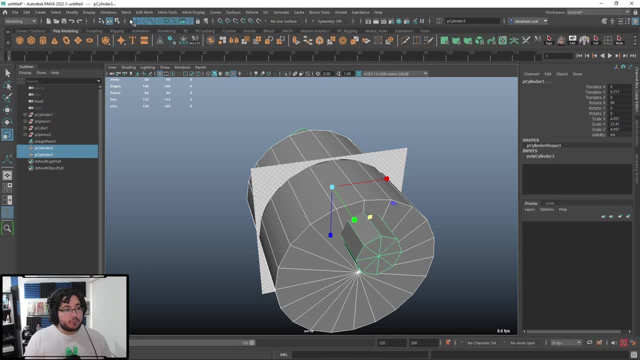 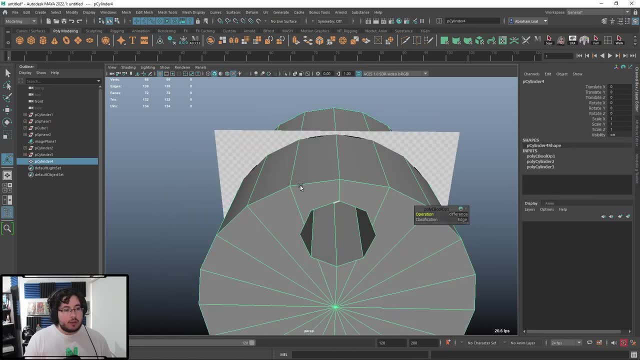 And then select this guy and this guy, And now I'm going to do a um, a mesh bullion difference. So what this will do, as you can see, it just created this whole uh, which is going to be the basics of this, like a pizza shape that we have here, which is what I want, uh. 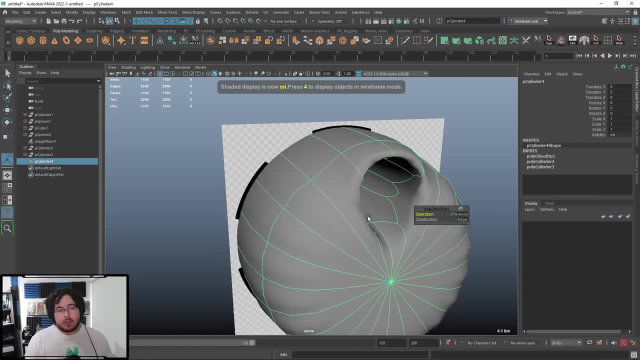 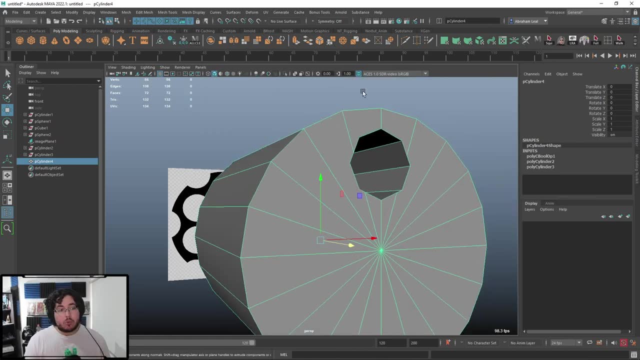 ready to to to work right. The problem is the topology sucks And if I try to do a smooth subdivision, it's not going to work. but here I'm going to show you how you can actually use a bullion to subdivide this in a better way. So I'm going to grab this guy. 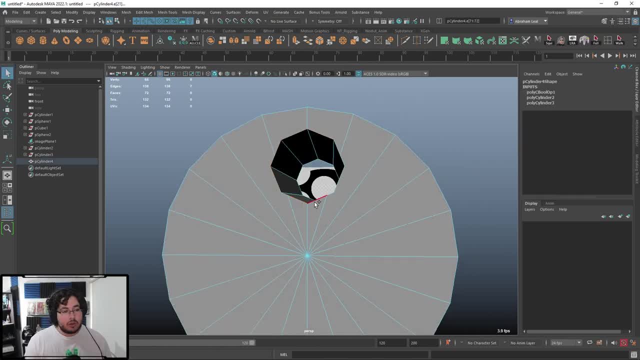 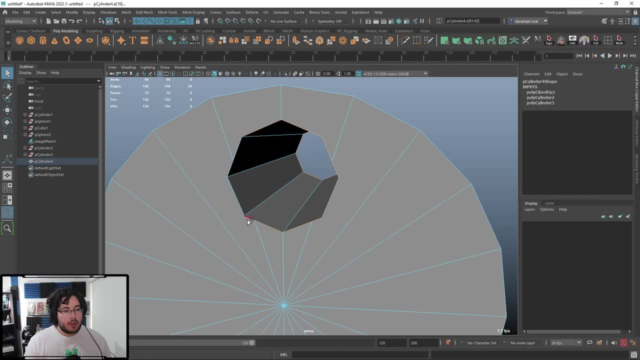 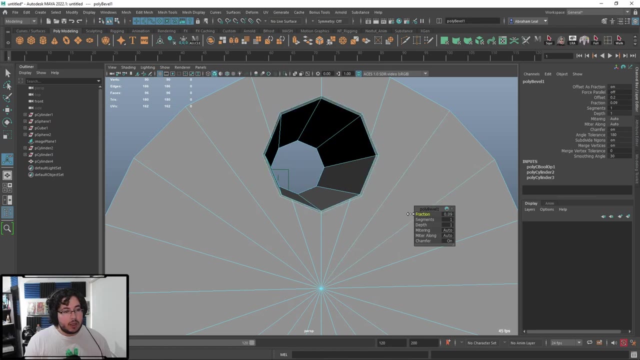 right here, And I'm actually going to grab the whole edge loop on both sides, like this: There we go, And by grabbing both edge loops, I'm going to, uh, do a, a bevel and or actually, sorry, sorry. Before that, uh, what I'm going to do is I am actually 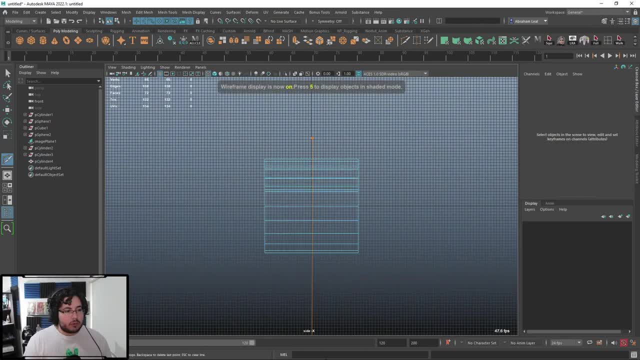 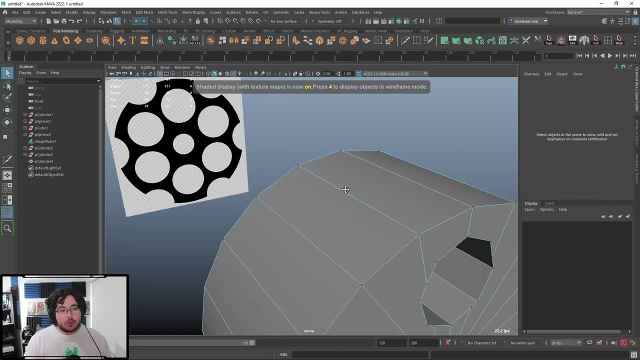 going to go to the side view. I'm going to create one cut tool right down the middle and then delete half of it. Why? Because it's easier to just work on one half and then fix the other one. So I'm going to fix the topology. I, I was, um, I I'm, I was wrong in trying to do this. 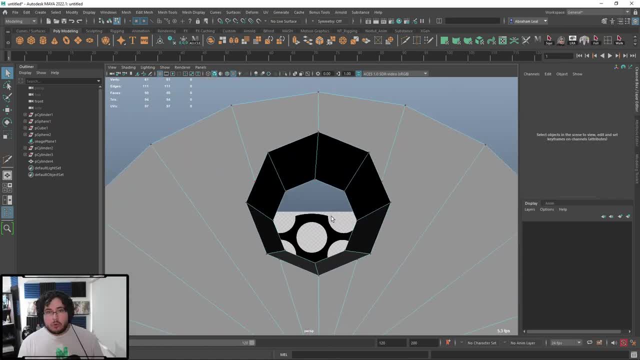 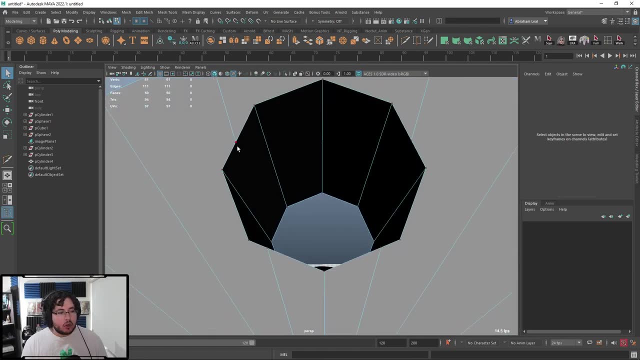 with the bevel. first, We first fixed the topology, and we already know- we saw that yesterday- that we need to have triangles and squares. As long as we have triangles and squares, then everything's going to be flowing in a in a better way. So right now we have this. 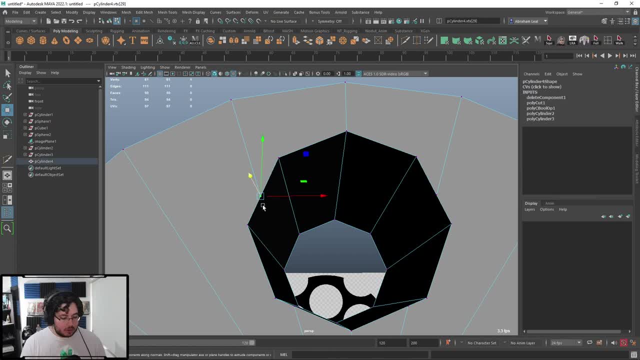 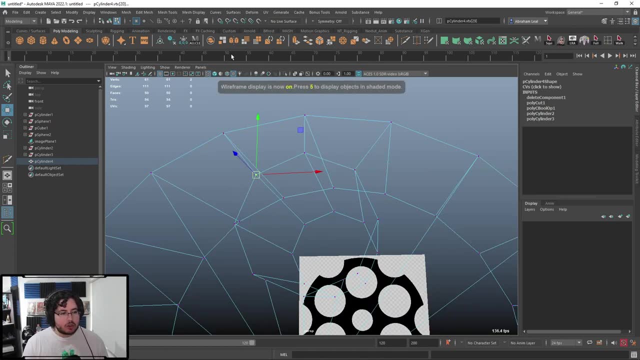 point right here, though It's not exactly where I want it to be. So if I go into points and I just snap this up here and grab this guy and snap it up here, you can see that we pretty much fixed the issue up here, because we can just grab this. two guys combine them. 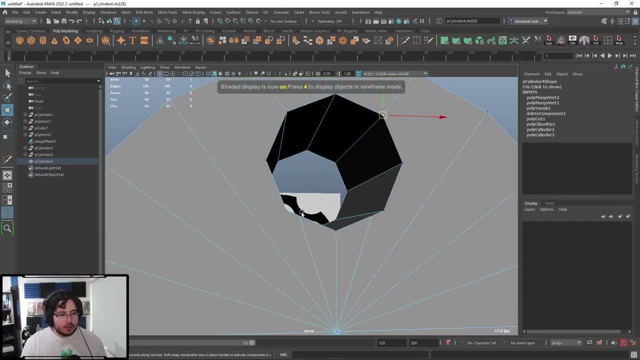 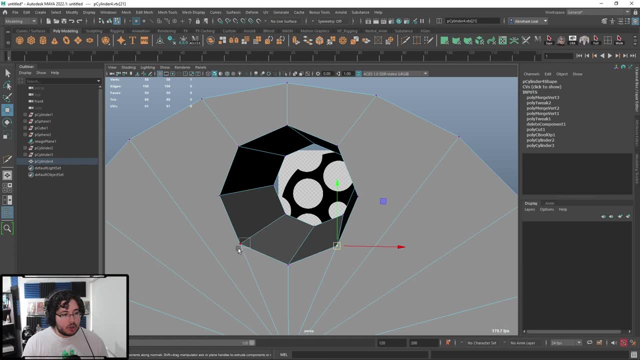 grab these two guys, combine them and then the topology is flowing in a in a in an even better way. We can do the same thing here. So B go there, here go there, grab those two guys, merge this two guys and merge, And now again we solve the topology in here. 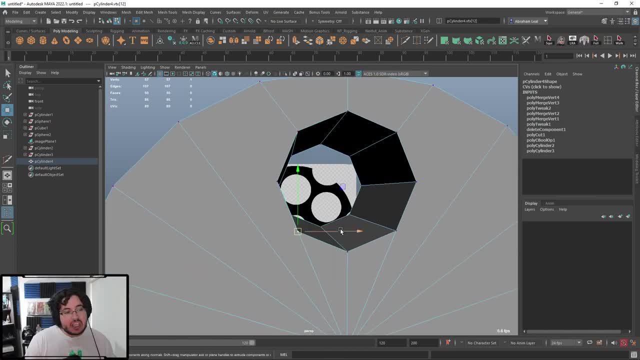 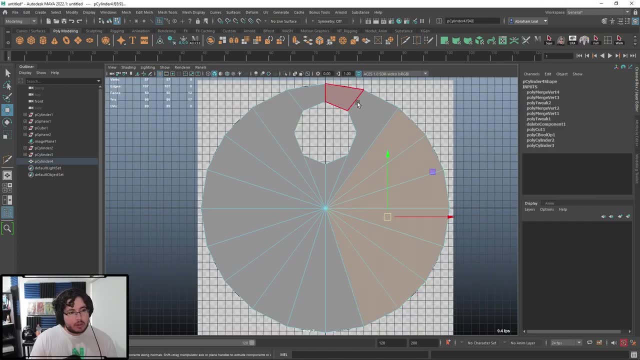 which not perfect because we have this triangles, and triangles are finicky, uh, but better, Uh. now I'm going to go to the front view, actually, and I'm going to delete all of the other faces here, because these are four faces And I know that if I got over this four faces- 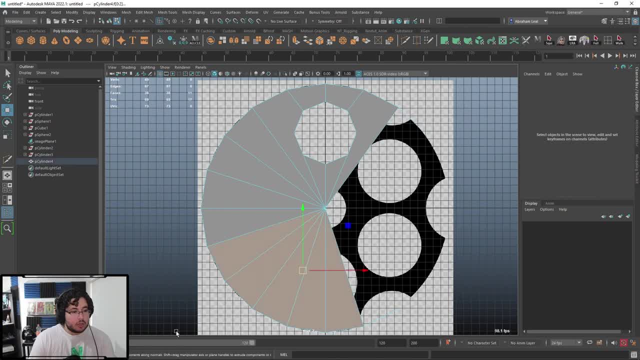 and multiply them five times, I'm going to get the four faces. I'm going to get the four faces in the whole circle. So I'm actually going to just work on this four faces right now, which again is: it's another one of those things that you need to take into account. 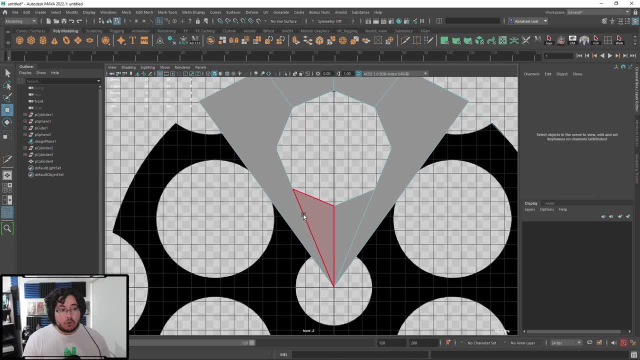 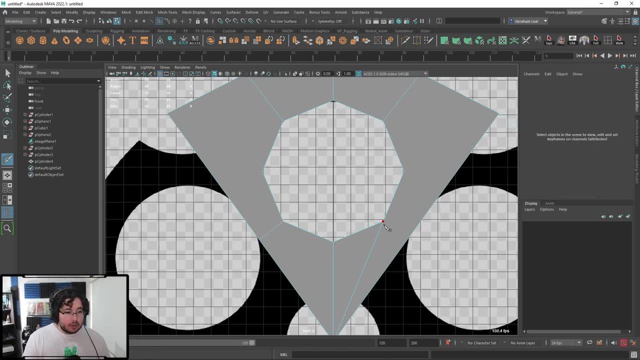 to make sure that, uh, you understand how topology flows, because we don't want to do any extra work Now. I'm going to grab my cut tool. I'm going to go from this corner to the border right here, And I'm going to go from this corner to the border right here. 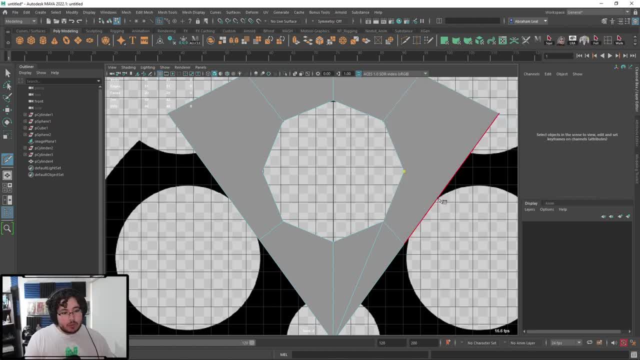 So what I'm doing there is I'm creating a new edge flow, or a new edge loop that I'm going to be able to just move like this way. For instance, here I'm also going to go like to the side, like this: 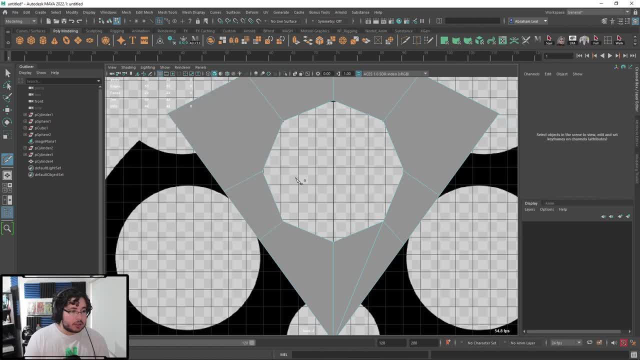 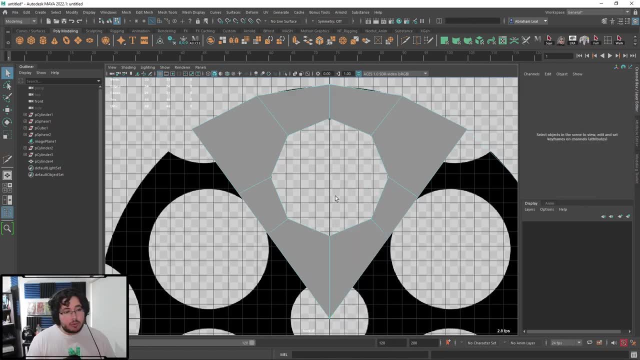 And then from here I'm going to go to the side like this: Okay, And that's going to give me, as you can see, squares pretty much everywhere, And I can actually delete this guy right now, this edge loop, and we're going to get square, square, square, square, square. 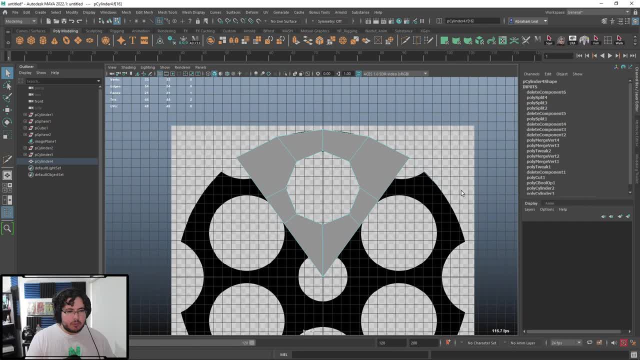 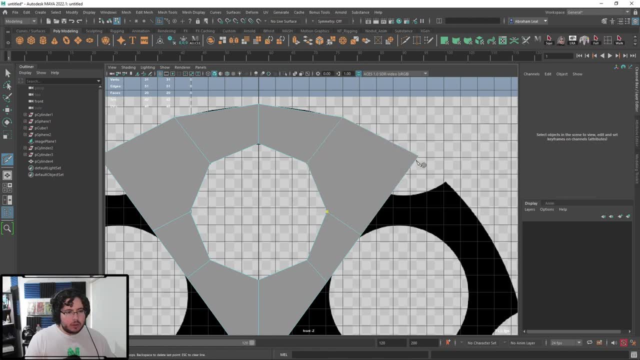 and then a couple of angles. Now, those angles I'm not really worried about because I'm going to be fixing them, And the easiest way to fix them is to create another little, uh like edge loop going to the corner right here. There we go, So from here to here, because 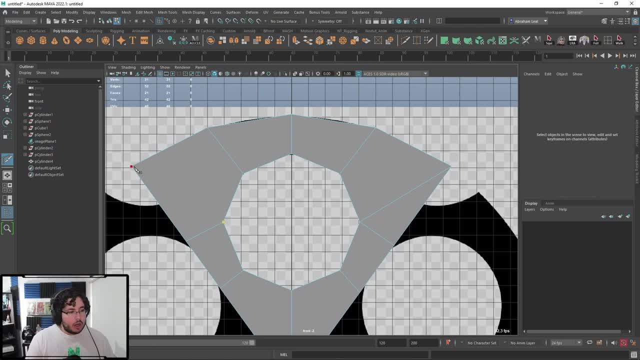 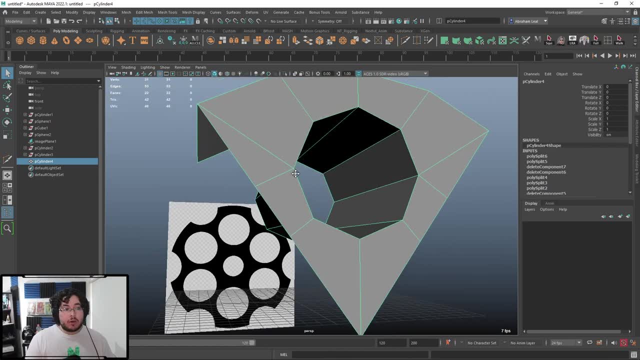 we, we do not want to modify the curvature of the of the outer edge, So something like this: And now, if we were to smooth this out, as you can see that the smoothing works a lot, lot better. Here's where I'm going to do the bevel now, because it's going to be. 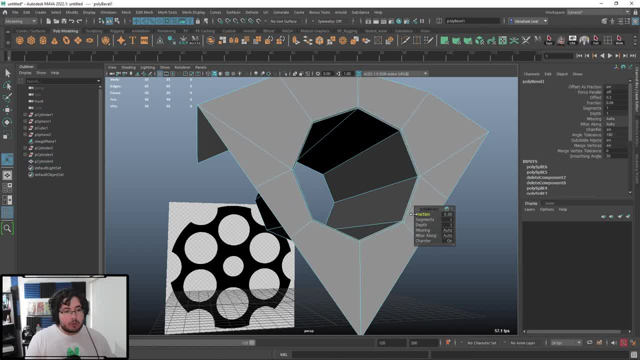 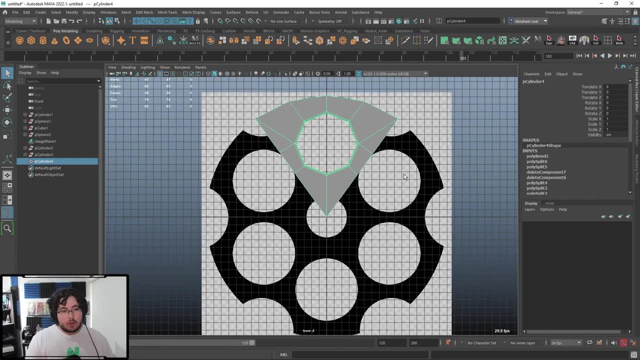 easier to just grab this whole thing. do a small bevel, small fraction, Let's do two segments And there we go. So we have this, uh, uh, initial part of the gun. Now to uh properly, uh, duplicate this thing around. What I'm going to do is I am going to um. 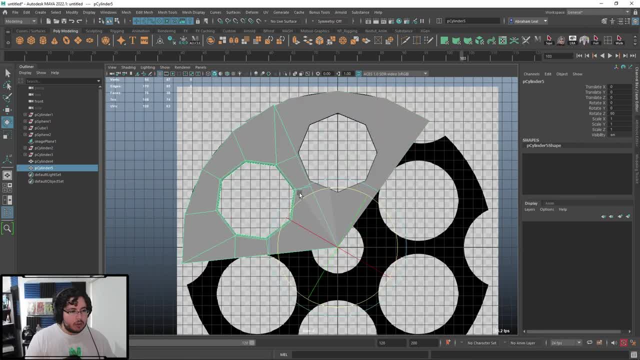 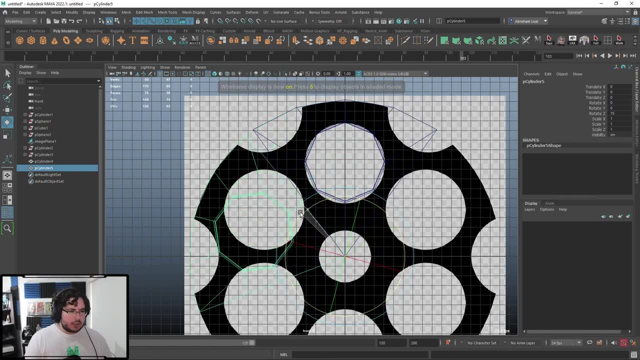 grab this, This guy, move it around, And if I move it like this, you can see that we're going to get, uh, this sort of effect. However, it's not section not giving me the exact measurement that was going for, So let's try a different approach. I think we're going to have to get. 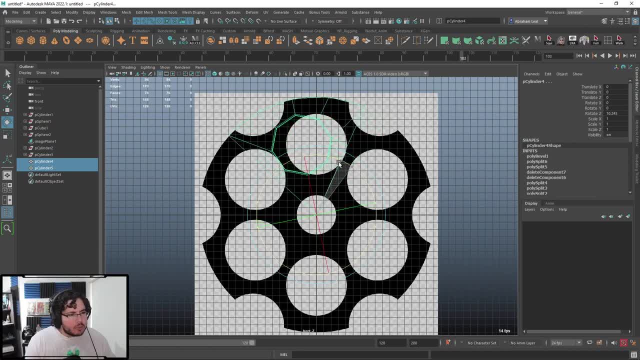 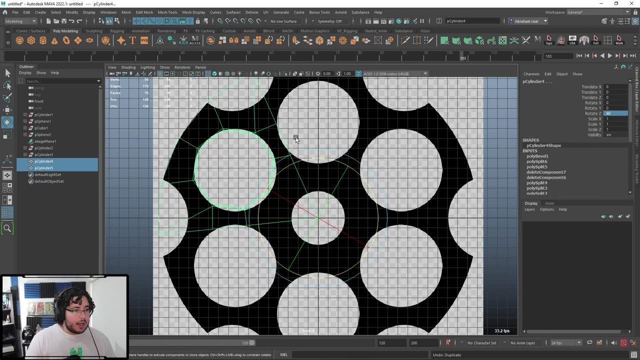 rid of, uh, discrete rotate, and the rotation is going to be, uh, about 60 degrees. I think 60 degrees. So there we go, Oh, 60.. As you can see here, let me uh bring this back. Uh, we're going to find this this exact. 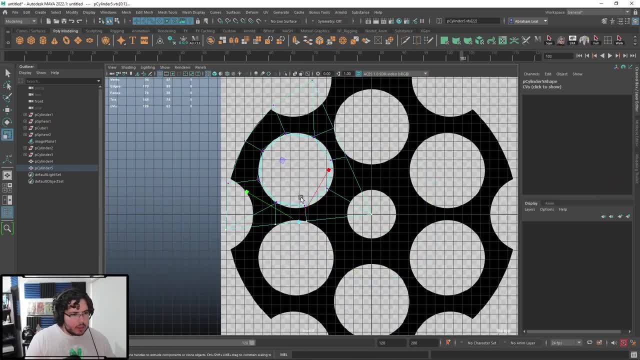 point. Now, what I'm going to do here is I'm going to grab all of this vertex and I'm going to snap them, uh, to world or to yet to world, because I think we're we're not exactly oriented the way. we should give me just one second, Not this one, this one. let's erase that one. 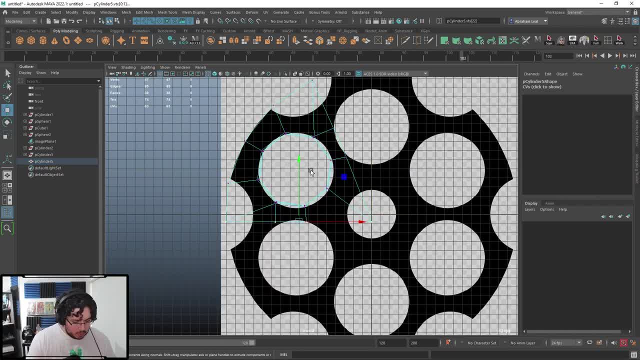 So this, guys, the thing that I want to keep the most consistent is the upper part. So there we go. So I'm going to go there And then I'm going to bring this thing back to zero, because this is the proper thickness that I need. So I just that rotation to find the proper thickness And then I'm going to. 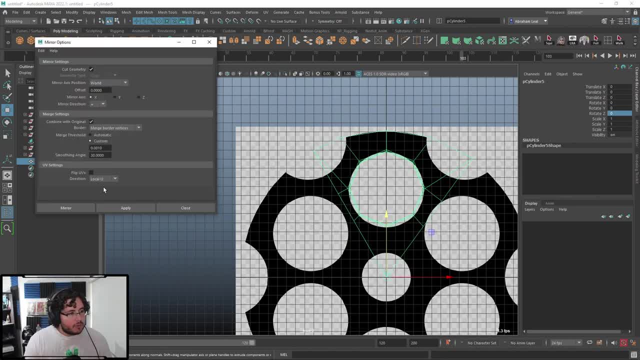 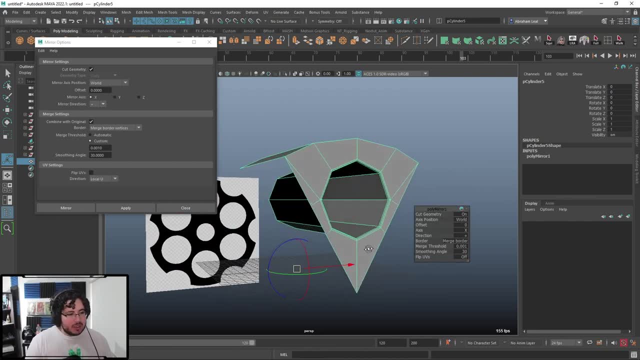 mirror this thing on the positive X. Sorry if this is a little bit confusing, kind of like freestyling right here. Uh, so yeah, there we go. And now we've pressed number three, As you can see that the apology, it works a lot better. And now, since the proper 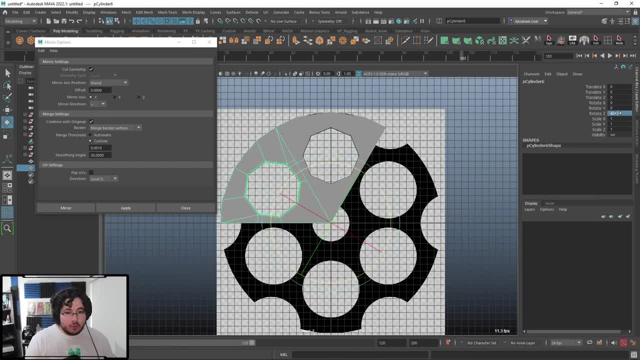 segment is working here. I should be able to just duplicate this thing, rotate it 60 degrees, Uh, like here, and we'll get this. and we can do the same thing. Just add more, 60, more degrees, So 120,, uh more. if you're bad at math, you can also use an operation here, and it should. 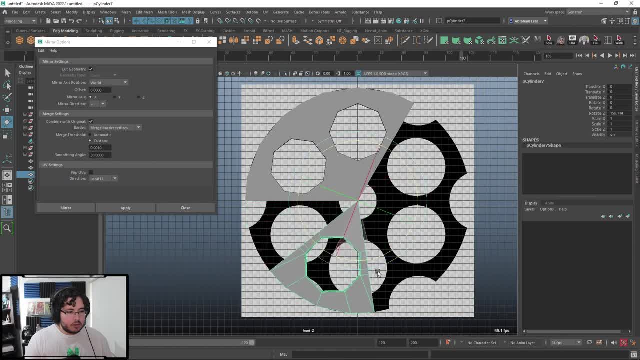 give you a yeah, so 120 plus 60.. That's not giving it. That's weird. I tried earlier in the work, or was that blender? I think it was better. I think blender has the math on the elements here. 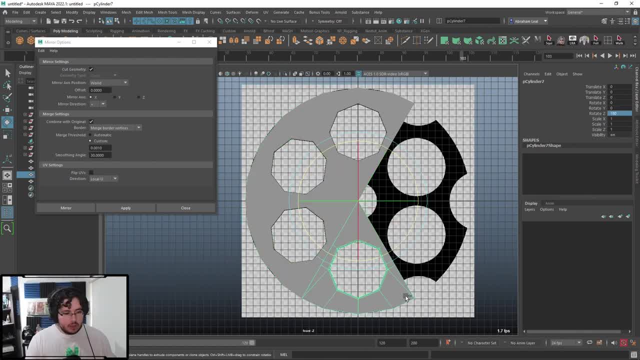 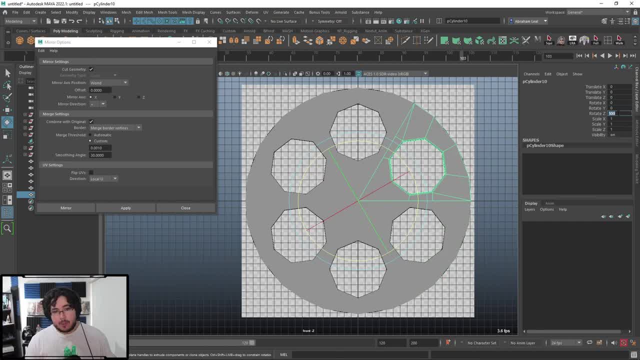 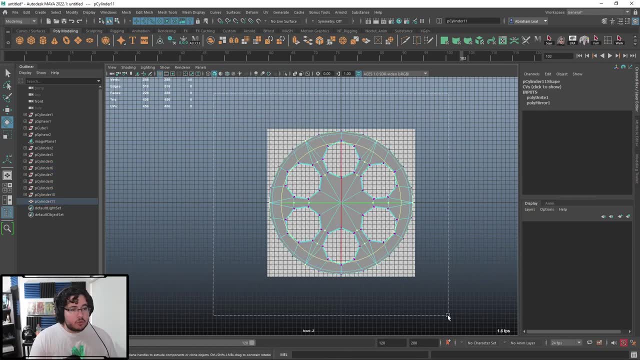 And then finally it would be 300.. There we go. So now we can grab all of them, all of the pieces, combine them into a single object and then go into vertex. grab all of the vertex and say mesh, or edit, mesh, merge. 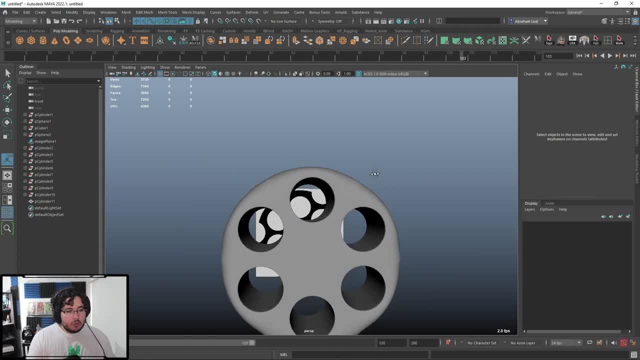 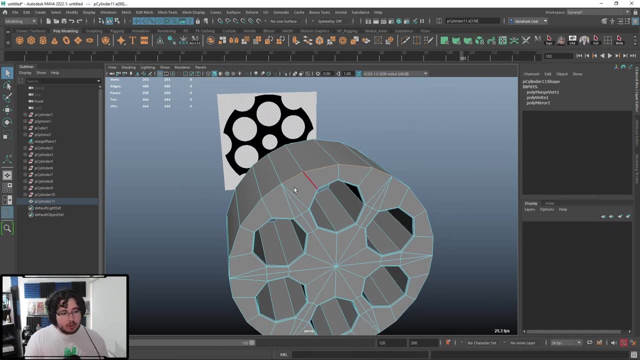 And all of the vertices that are in the same place will merge together and, as you can see, we're gonna get these very nice chambers. Now, of course, we have the issue with the upper part, where this thing is not working properly, as you can see. 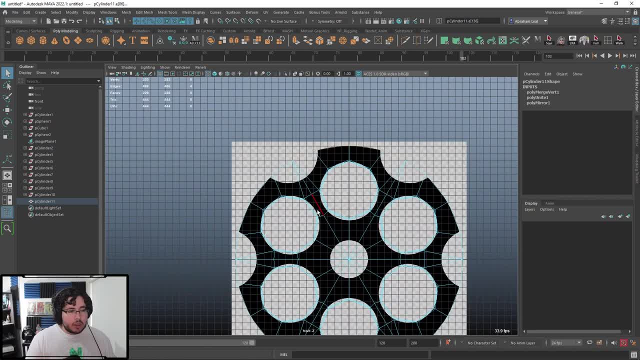 but we're gonna fix that. So, now that we know that this is gonna work, we need to find this thing right here. right, We need to do the little hole, and we're gonna be using another Boolean to do so, and this Boolean's gonna be a little bit more interesting. 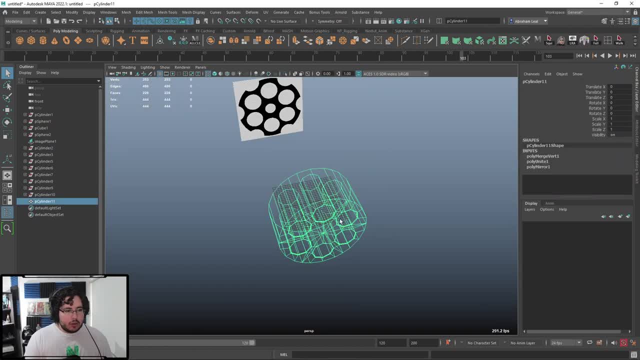 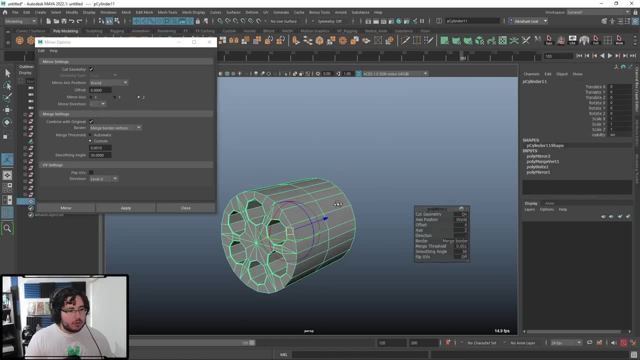 So what I'm gonna do is I am first gonna grab the whole object and do a mirror to C, C, negative, so like this: hit apply. there we go, so that we have the other side of the barrel, And then I am gonna go to the front view. 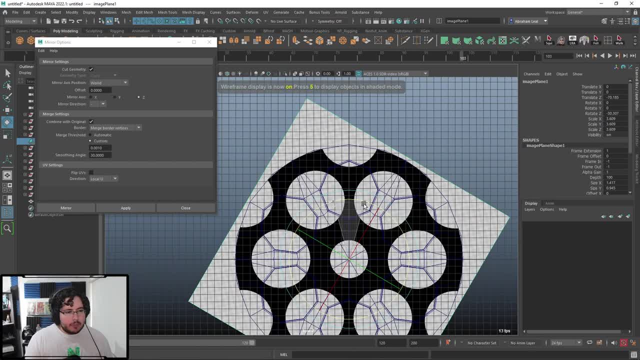 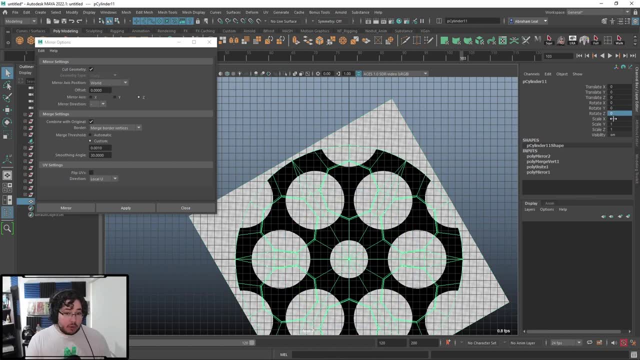 grab this guy, and I believe we need to rotate this about 30 degrees. so I'm gonna say 30 degrees so that we can see now that line right there, which is what we're gonna be aligning everything with. We're gonna grab this guy, of course. 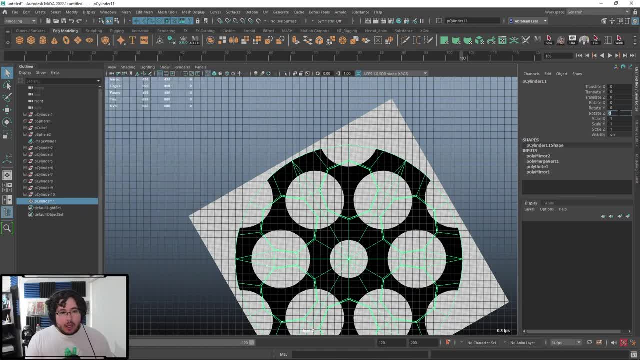 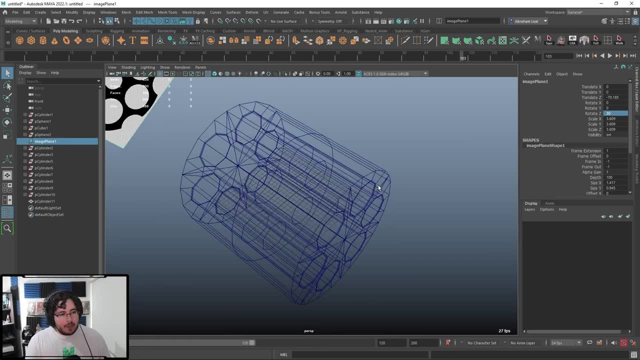 and we're gonna center the pivot point and we're gonna rotate this thing 30 degrees as well in C, so that the holes are aligned with everything else. Now I know from the times I've done this exercise that this cut right here does not go all the way through. 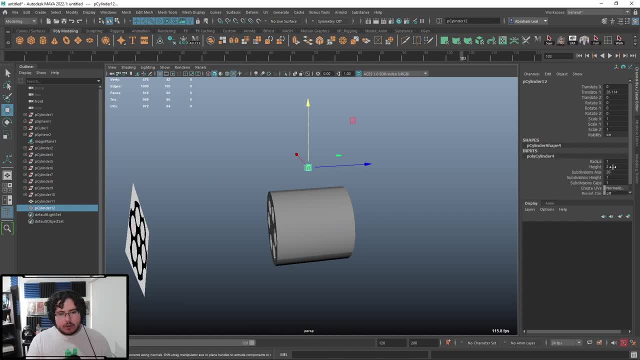 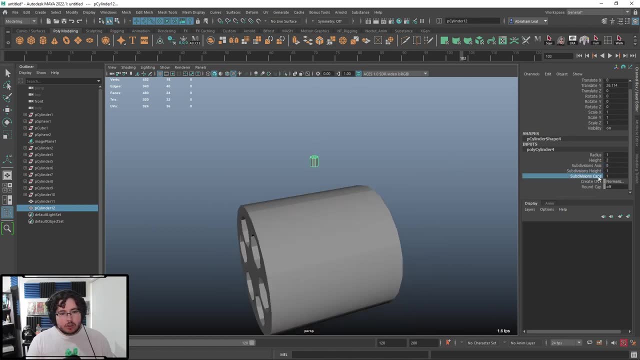 so I'm gonna start with a cylinder. I'm also gonna make the cylinder eight sides here real quick, and we're gonna do subdivision heights, subdivision caps- sorry, I'm gonna say three- and then round cap I'm gonna set on. 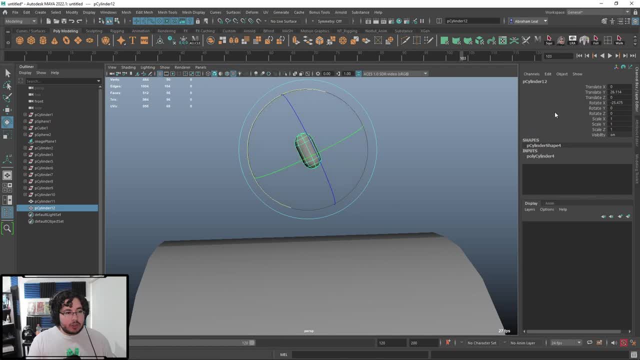 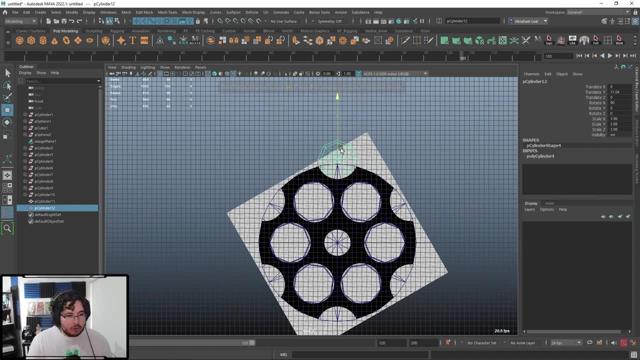 and that's gonna give me this sort of like a pill. So now I'm gonna rotate this pill so that it's 90 degrees facing me, We're gonna go front view and we're gonna scale this so that we create the hole or the circumference. 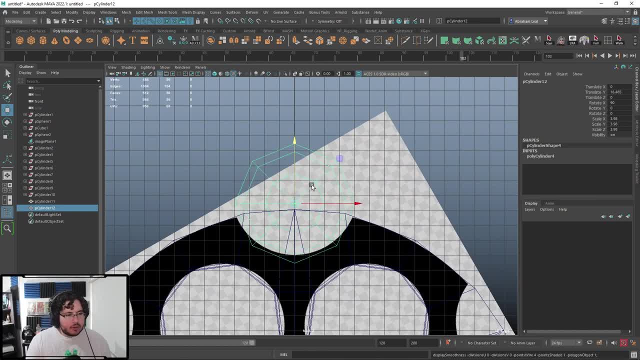 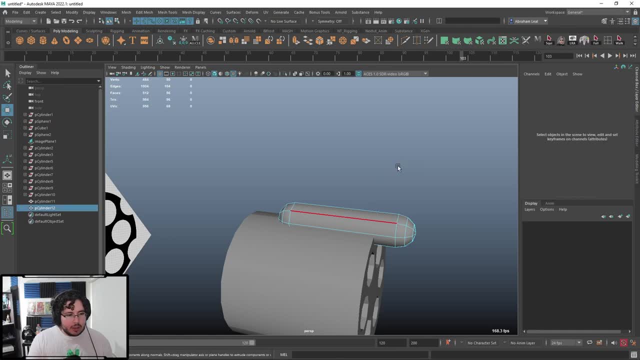 of the hole that we need, which is about there. Okay, Yeah, about there, there we go, And now the only thing I need to do is I need to grab all of this front vertices and push them forward so that this shape is gonna cut into this shape. 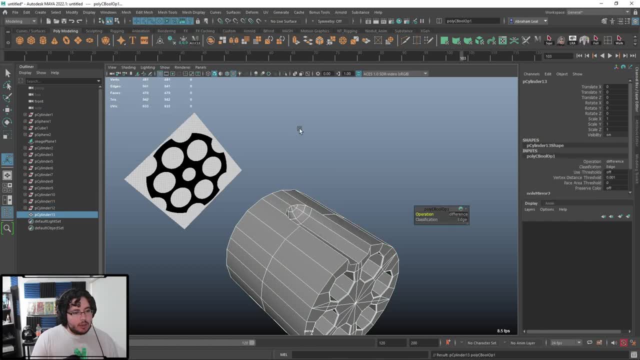 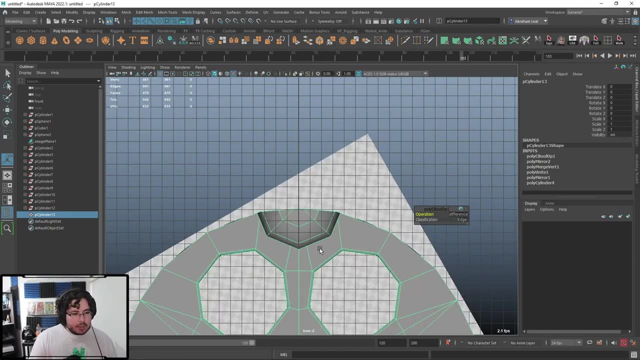 So we grab this guy, this guy, mesh booleans and difference And, as you can see, we do get the cut that we're looking for, but it's not how we want this to be. Now the cool thing is again. 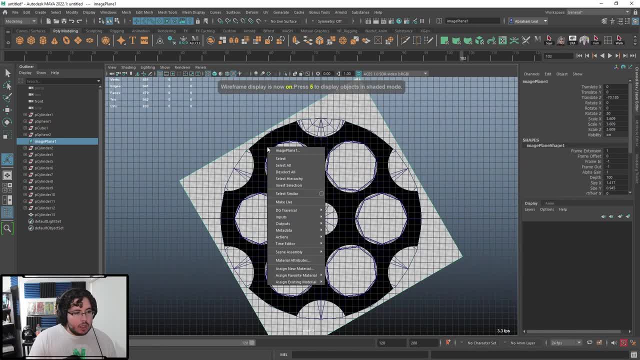 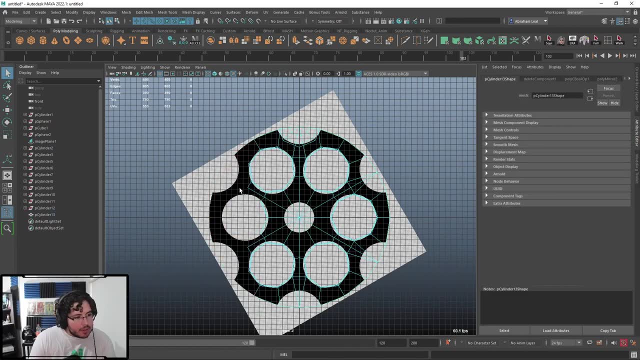 we don't need to worry about all of the other cuts because eventually what we're gonna do is we have already this sort of like pizza slice. so if we grab, like this half right here, the sort of like triangular shape and we just eventually mirror it back, 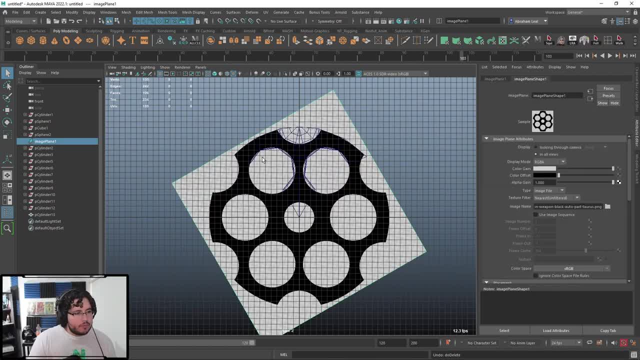 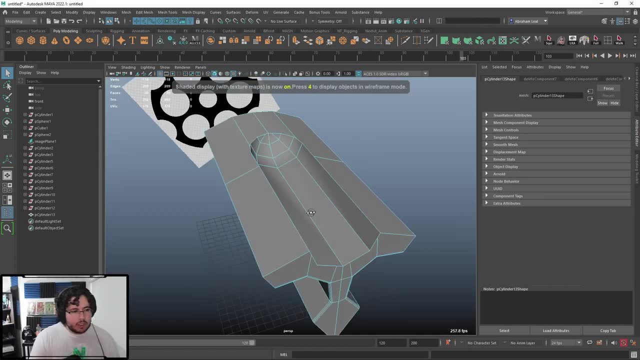 like a, like a T-shape- There we go and this guy- there we go. So if we mirror this thing like several times, we're gonna get the exact thing that we're looking for. So it's easier to just fix this area. 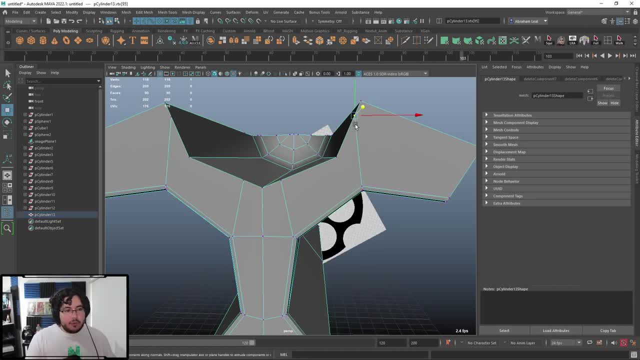 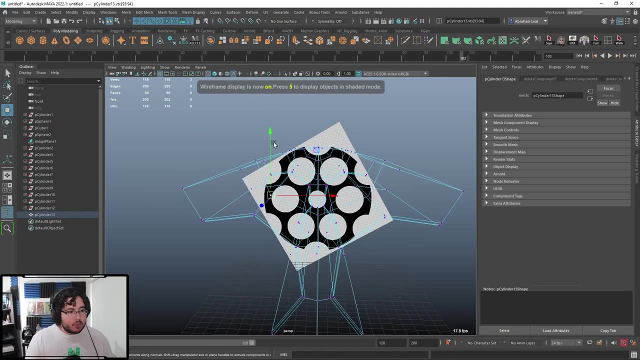 than to fix the other parts. So remember that weird triangle that we had before. Now it's very easy, because we're just gonna use this point right here, this point right here. i'm using v snap to point to snap it to the specific point we're gonna merge. 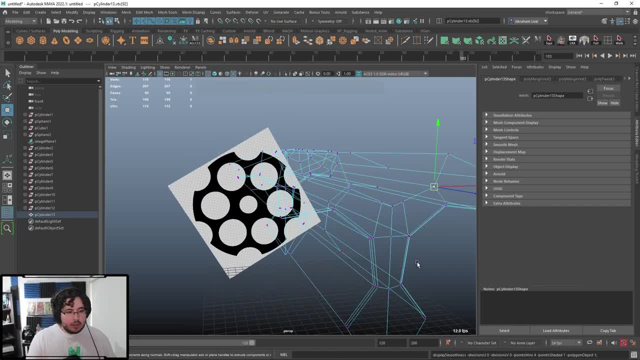 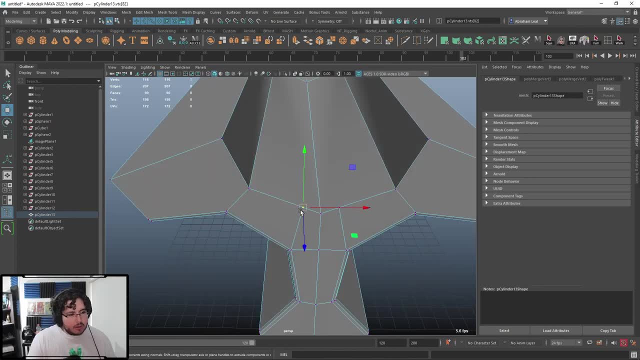 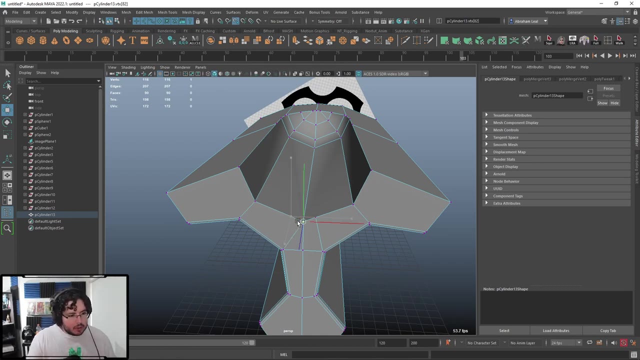 together and merge together and, as you can see, that thing is gonna get solved right there now. over here we still have a couple of uh issues like this guy right here, uh, and this guy right here now. in this case, i would say it's a little bit easier to, um, just snap it here in the center like this: 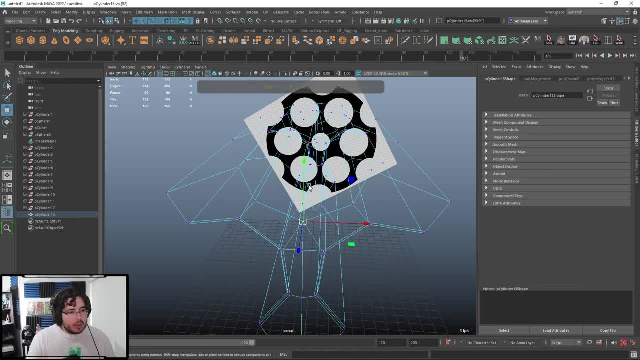 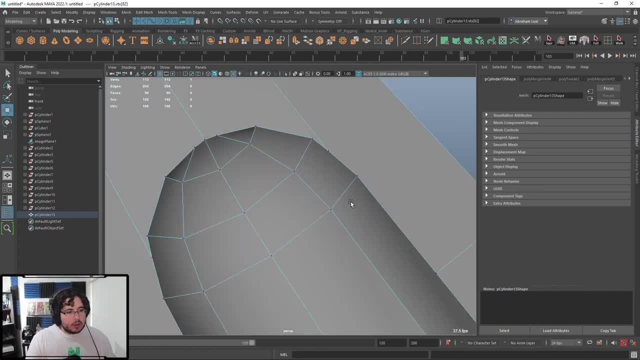 and like this, and then just grab those two guys and snap them together and that way we're gonna get a nice like sharp angle right there. now on this side, you can see that there's a lot of lines as well that are having a little bit of an issue. so i'm gonna- i'm gonna find where these vertices. 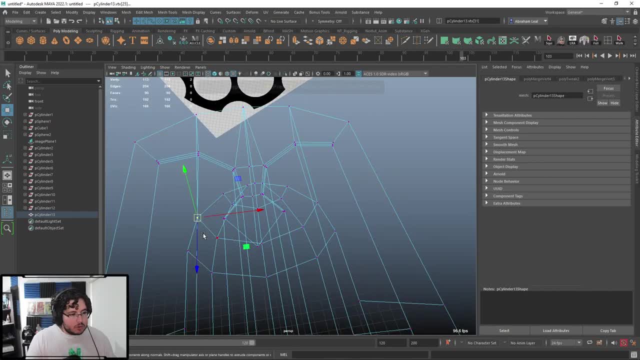 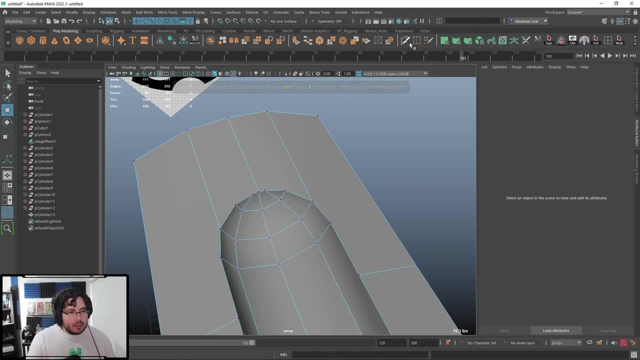 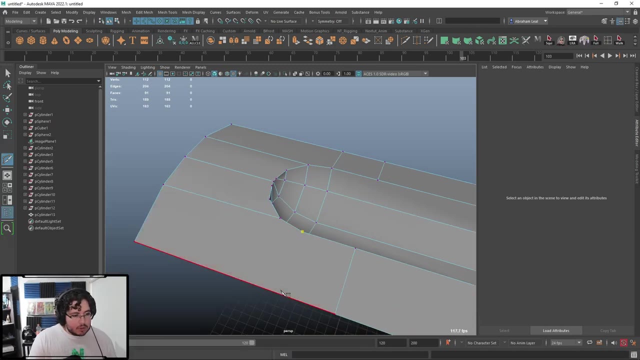 can just like point to each other like this: like those two guys are very easy to solve because we just merge them together and that makes a nice square flow. then from this side it's very easy. we just grab this guy right here and we just snap it to the side like this, and then we just grab this: 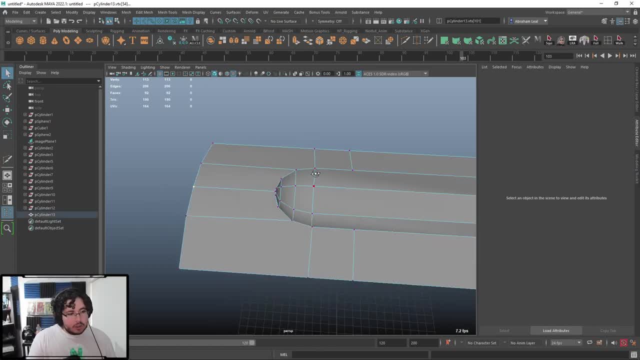 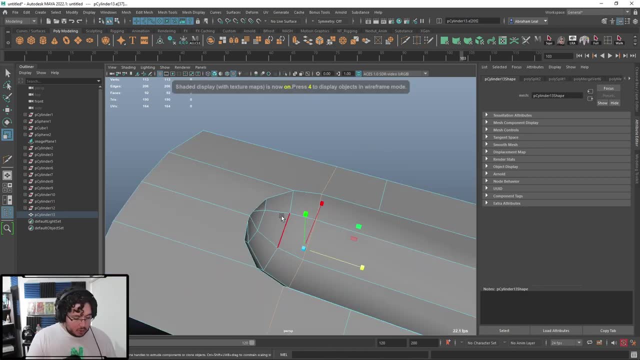 guy right here and we snap it to the side like this: you very important that we grab this edges, or this new edge that we just created, and with the r key we snap it together. so it's perfectly flat and we're gonna do the same thing here from here. 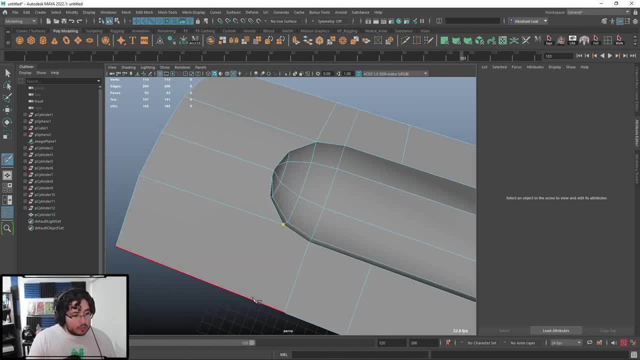 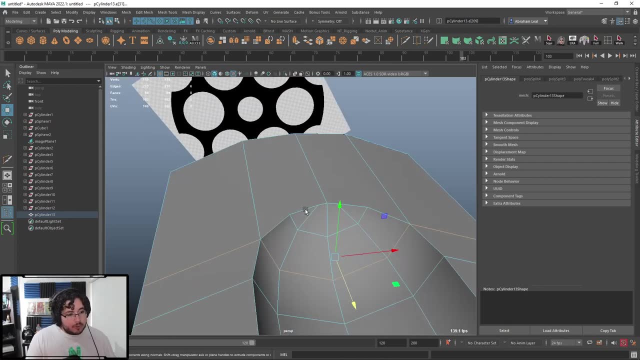 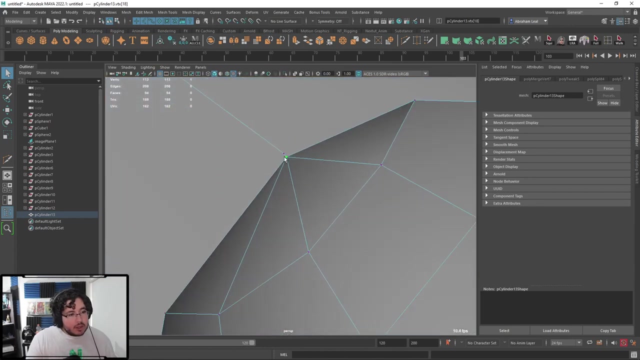 to the side and from here to the side. like this, we grab the whole thing here here r to to scale it and there we go now for this area. you can see that we still get some like weird elements. all of those guys i'm just gonna merge to center so we can create a nice triangle. you can see a little. 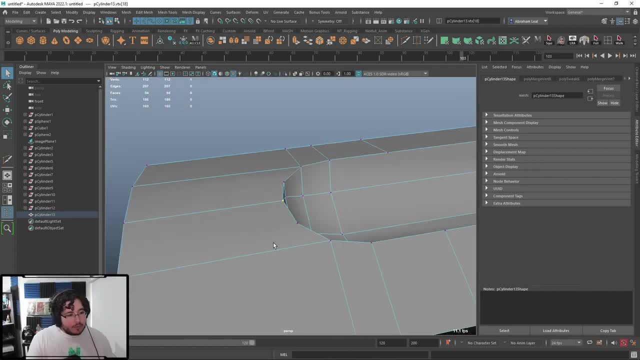 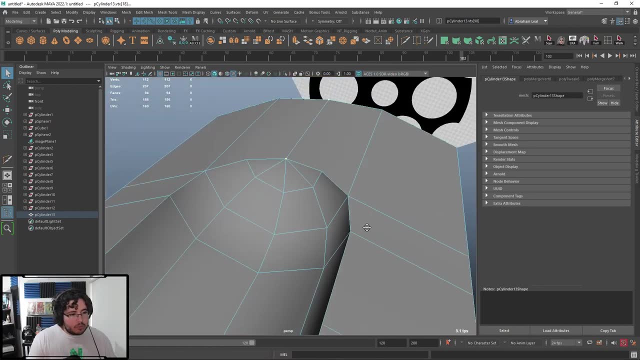 one right there also merge to center, and we're gonna do the same thing here, from here to the center, to clean it up. and then we have this. remaining two ones, uh, and in this case i think it's gonna be easier to uh, just probably just have another set of triangles. so i'm gonna go from this. 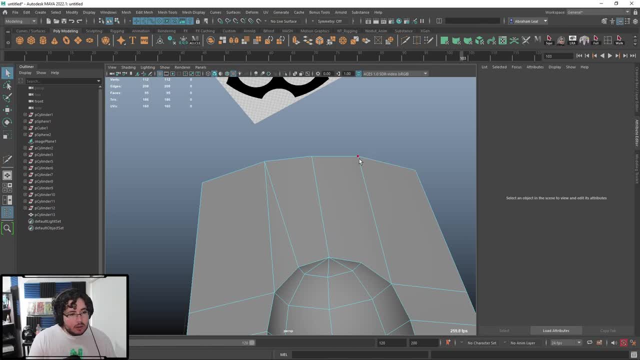 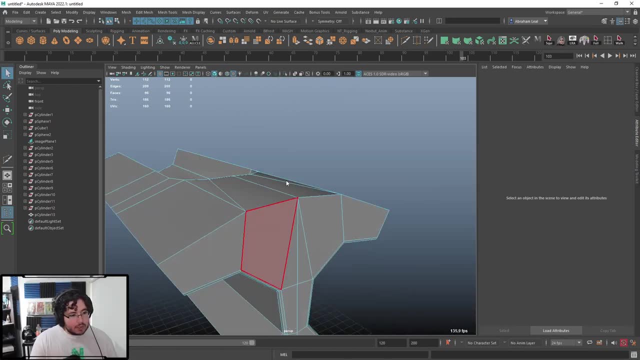 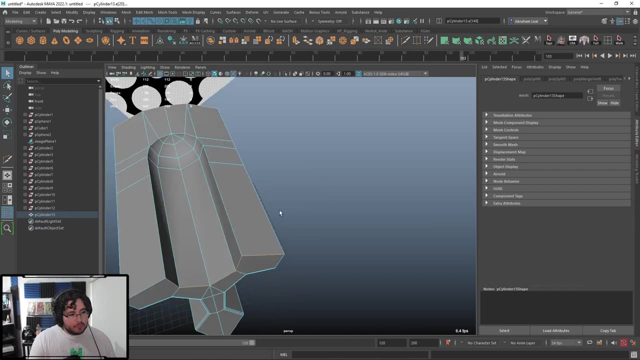 border to this border right here, and from this border to this border right here, there we go. so now we press number three. we have this very nice effect. now, this line and this front line, we're gonna bevel. actually, i'm actually going to bevel this whole line as well, and that bevel is going to help. 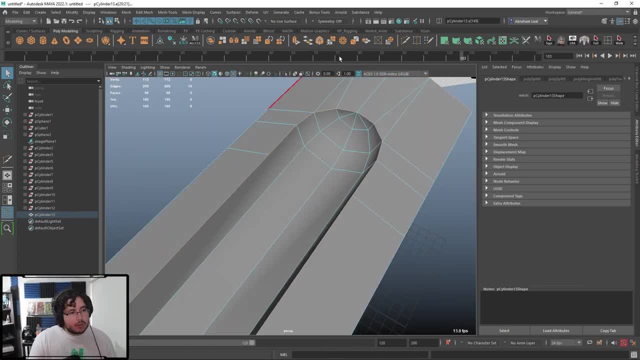 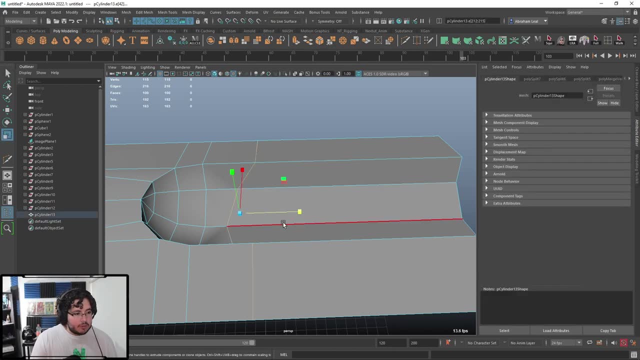 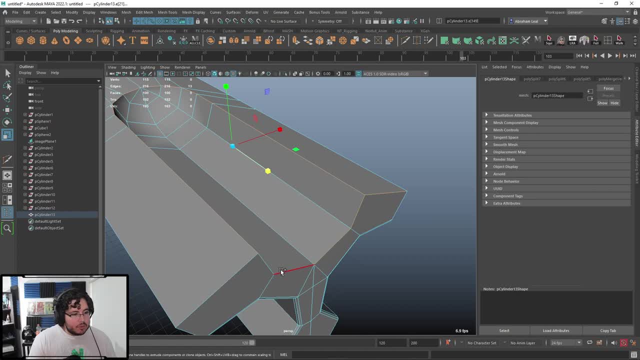 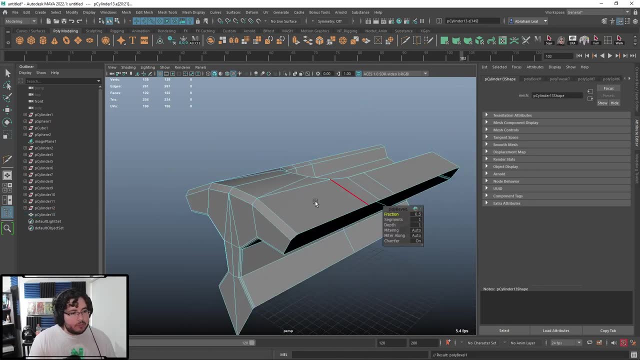 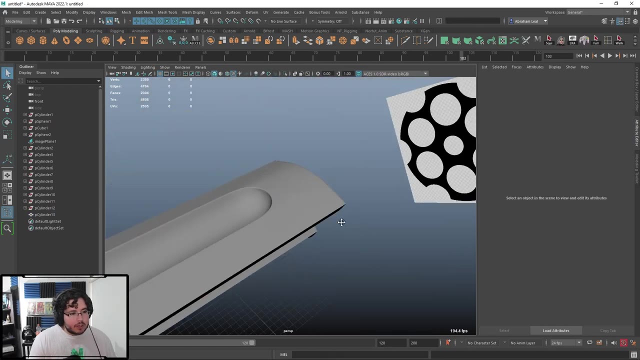 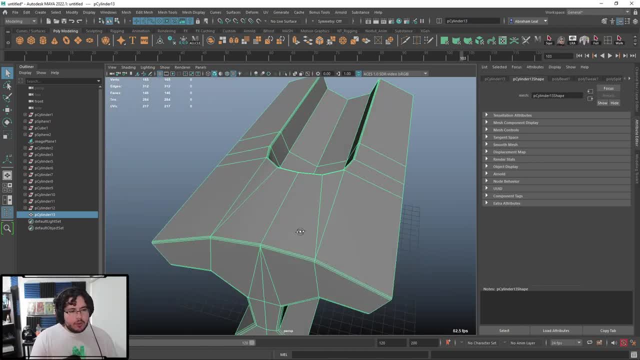 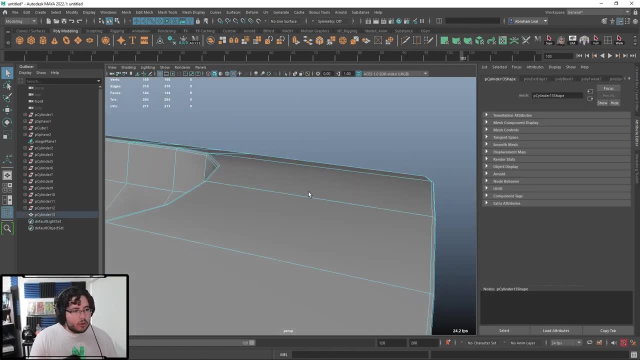 so there's, there's a lot of ways in which we can actually fix them. uh, one of them would be to actually like add another edge loop. we could also modify this edge instead of having it go to that corner. we could add: it's a little bit more, not super advanced, but just a little bit more advanced. 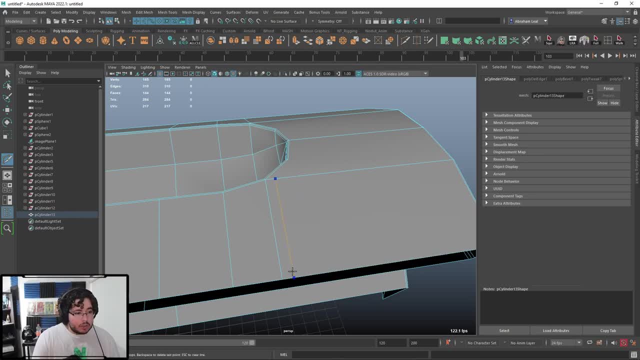 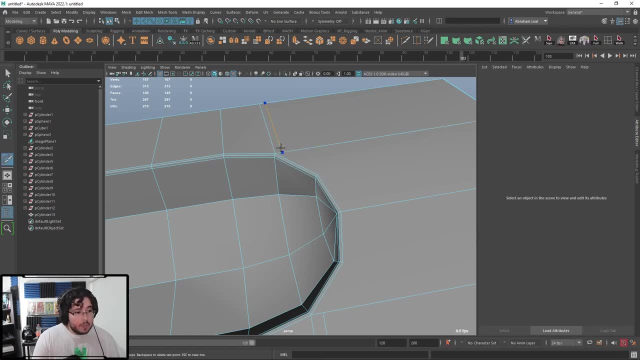 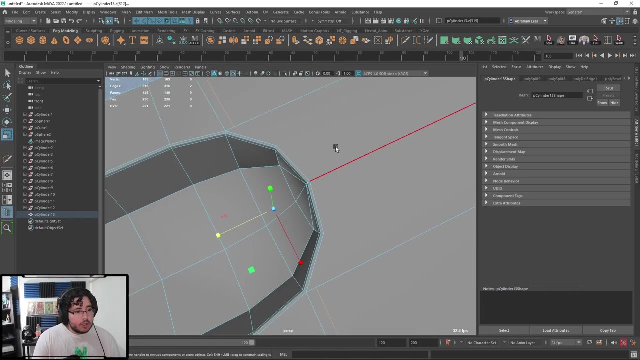 we could add another edge loop, like really close in here, like this, and then have the same one like over here. there we go. now this guy, because i want to keep them symmetrical with our key, i'm just going to snap them. there we go, and then i'm going to go from here to here, here, here, and then 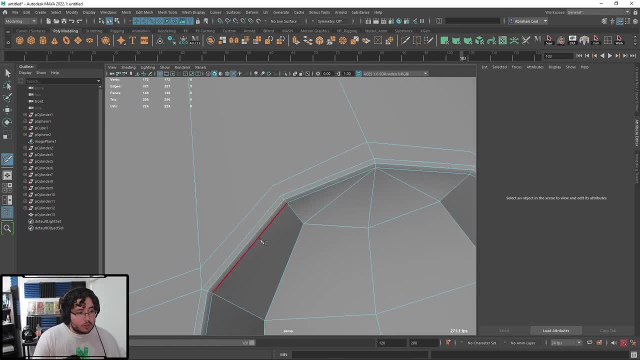 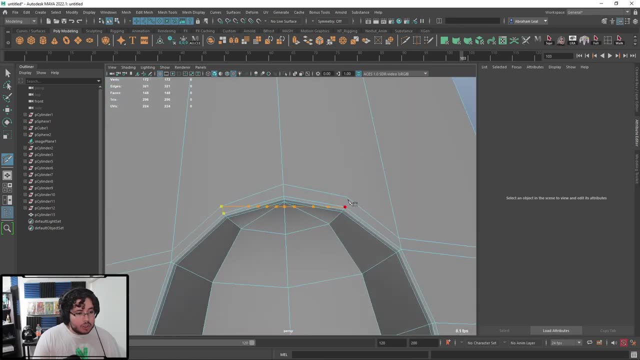 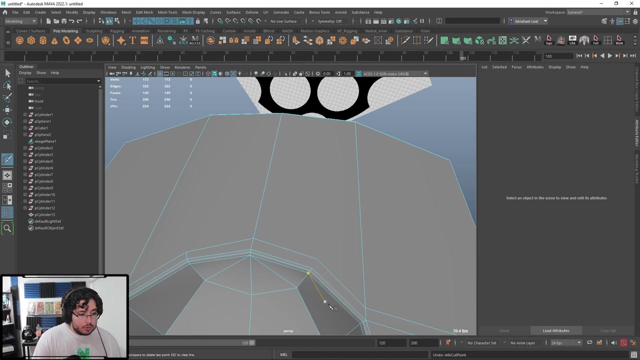 here, and that way, what we're going to be doing here is we're actually going to be creating a like like. we are going to create a little like pinch, but instead of having it go all the way over there, we're going to keep it really, really close here, so we're going to go. 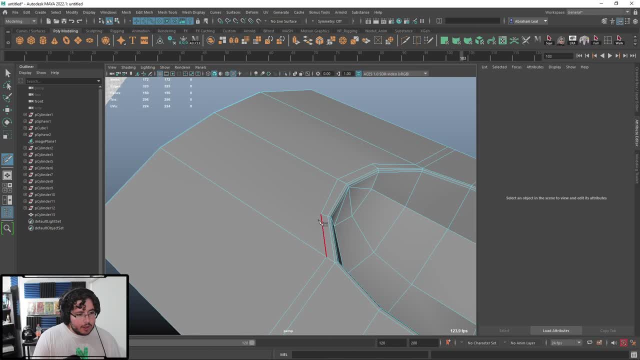 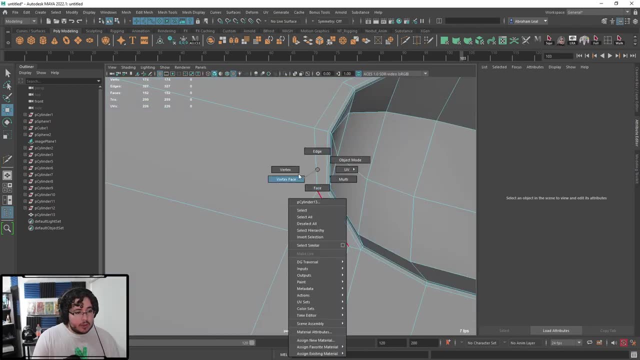 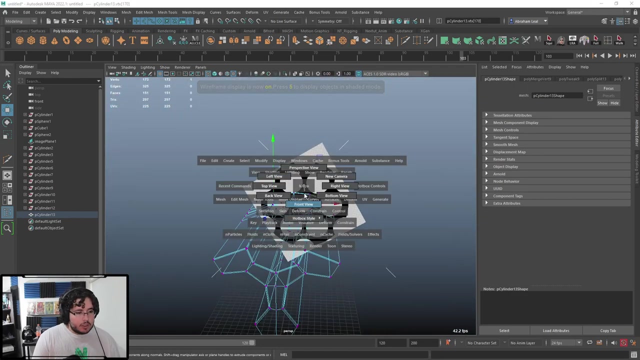 from here to here and and then we're going to move this guy, as you can see, to the side, like this. so we're we're moving the topology, and then this guy snap it right here, so those two guys merge together and actually this thing is asymmetrical as well, so we could just delete half of it. 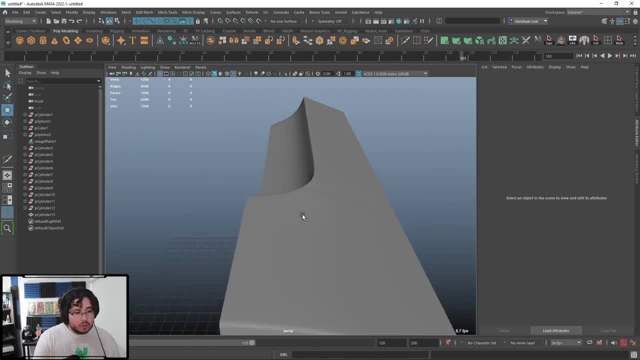 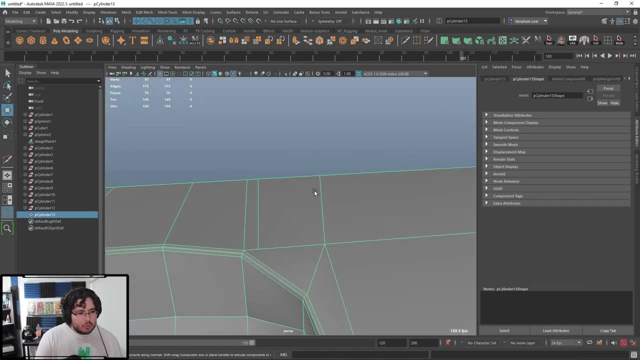 there we go and you can see we're going to get that sort of topology there, which is a square, but it's flowing a little bit better than what we have over here, which was like a weird pinch. you can see the pinch still there again, one way in which we can relax a little bit. 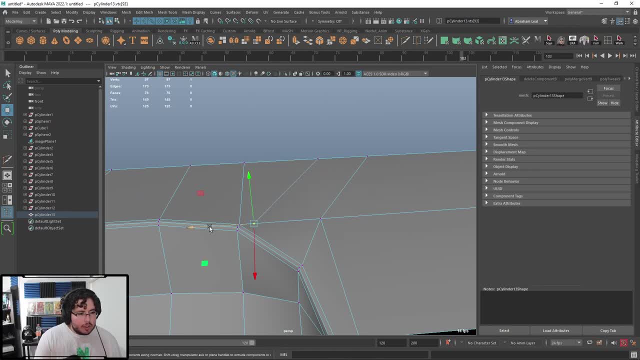 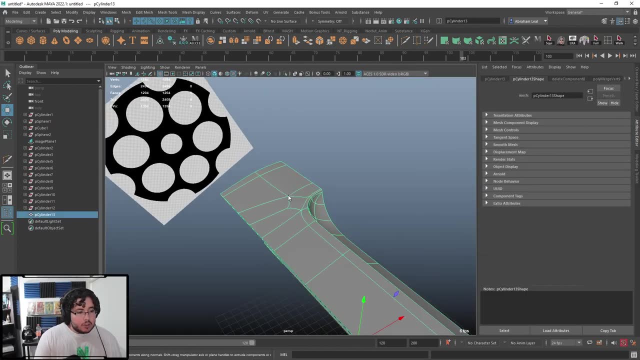 remember that the further away points are from each other, the the smoother they're going to be. so by moving the the points away, you're going to see that the pinch gets uh reduced quite a bit. so now we can just do this mirror to the uh x positive. 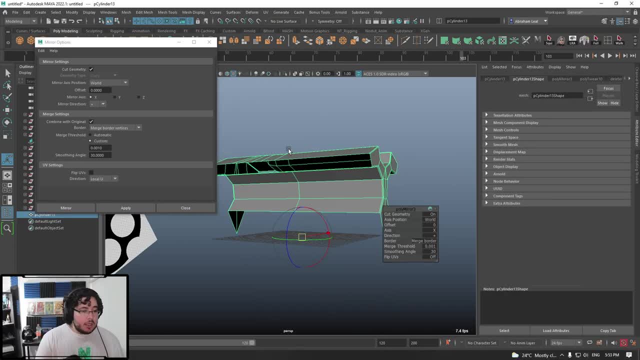 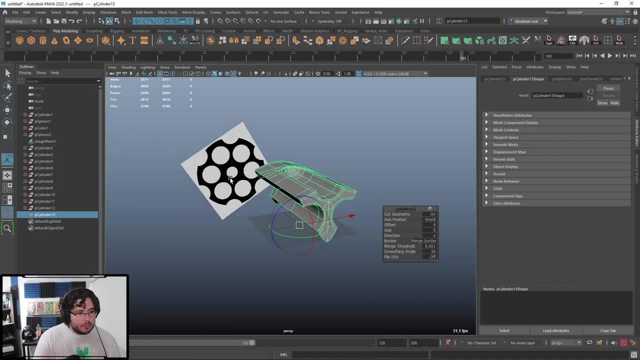 there we go and we have our shape and finally, i'm just going to use duplicate special, which is a very nice tool here, inside of uh, inside of maya uh, and duplicate the special will, um, you can imagine, duplicate this in a special way. so i'm going to go here, duplicate the special. 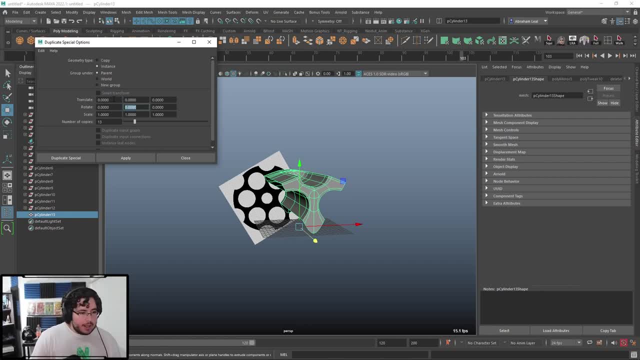 and i'm going to do a rotation which is going to be, uh, 60 degrees to rotation. so 60 the y-axis, and I want five copies because I already have the first one hit apply and no, sorry, it's in the c-axis. so 60 degrees on the c-axis, which is the 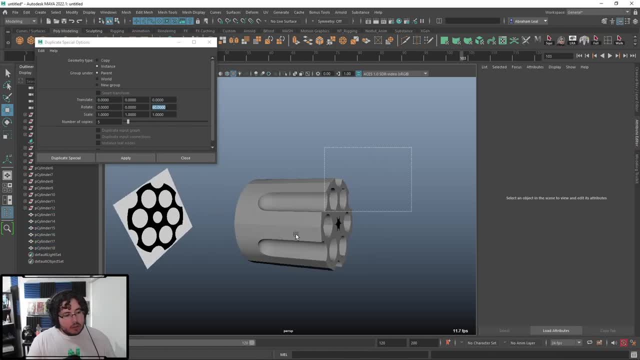 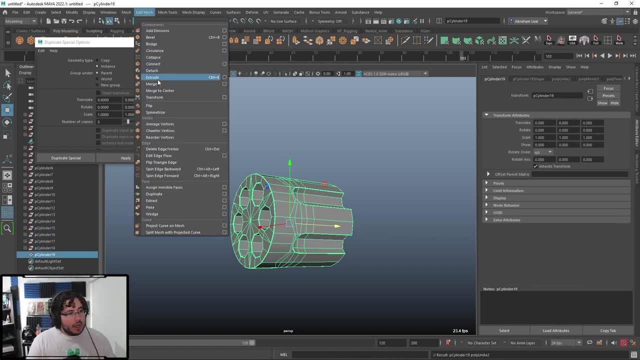 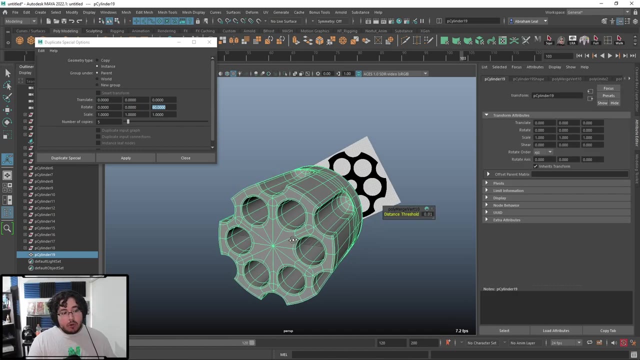 last channel and we hit apply, boom, there we go. so it's just a matter of grabbing everything here, going into edit, mesh combiner, sorry, mesh combine, edit mesh and a merge and, as you can see, we get this very nice element where we use booleans because, again, booleans are not our enemies. it's just a matter of 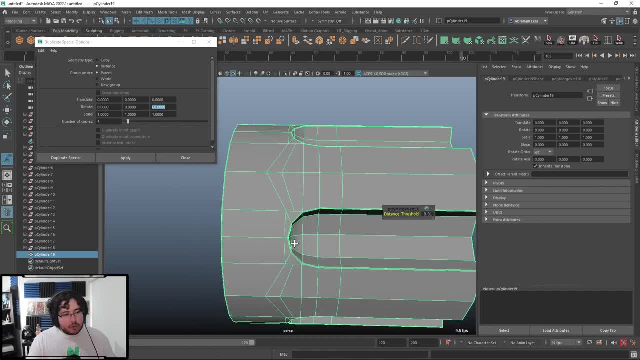 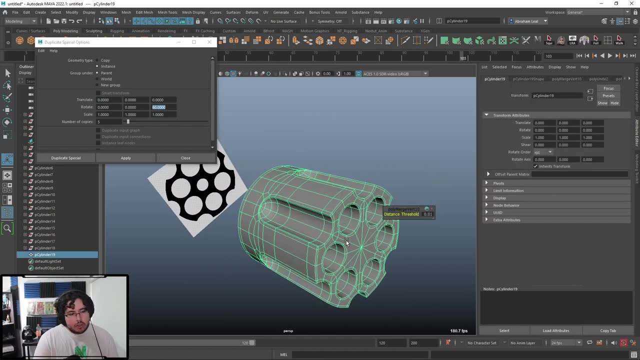 knowing how to properly use them and you don't have to go super, super dense. as you can see here, like this is a very nice topology, very, very low amount of topology, and you can texture this, you can UV this and it's, it's perfectly workable for games or for well, for games might be a little bit high, but for 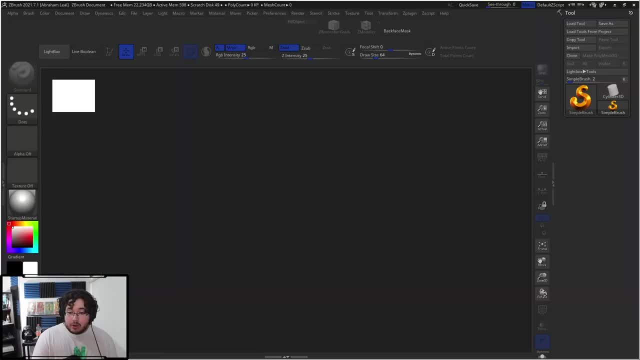 cinematics. it's perfectly fine. so that's it for today. guys. now I know that I opened C brush and I was gonna show you something, but I think we're gonna be running out of time, so we're gonna be taking a look at this tomorrow on.